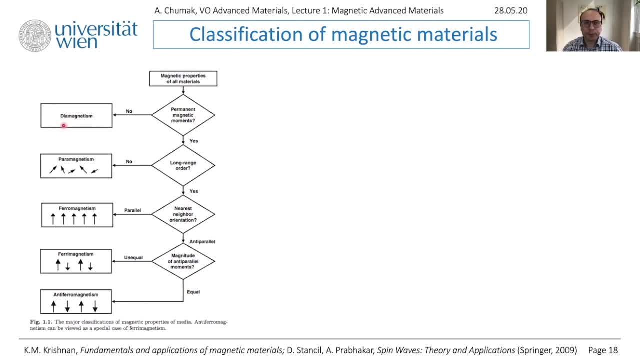 then you are dealing with diamagnets. If there are permanent magnetic moments and you need to check if there is a long term emitter range order, so if your magnetic moments are somehow filling each other or they are completely independent, if there is no order, that it's paramagnet, you say. 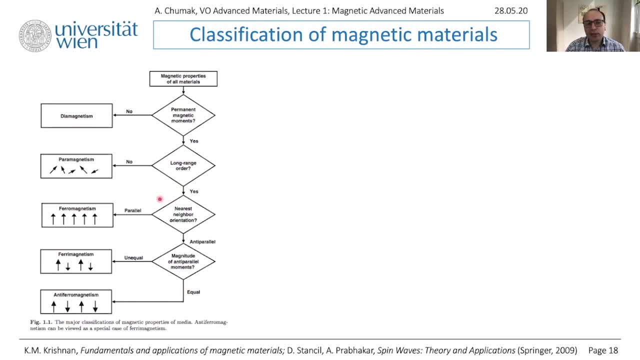 are filling each other, then the next question is: what is the orientation of neighbors? if they are parallel, then you're dealing with paramagnet. that's what we get used to actually in our everyday life. our magnet is some magnetic material, but there is also possibility when this magnetic moments. 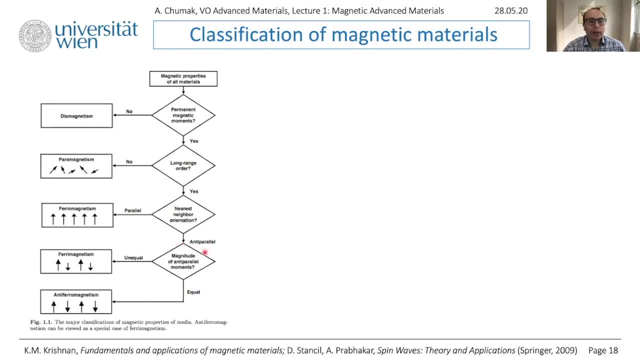 will stay anti-parallel. and then the last question you have to ask is if the magnitude of anti-parallel moments is the same for both sub-lattices or it is different. so if sub-lattices have one which has this magnetic moments point in. 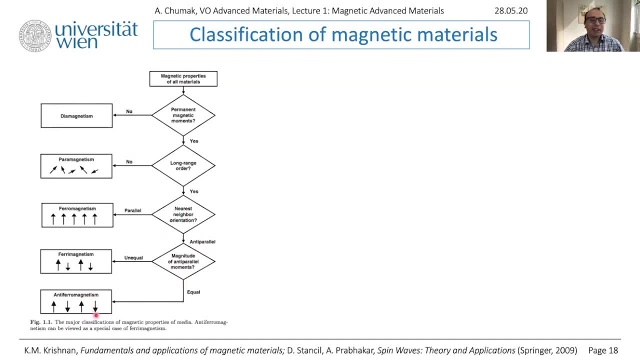 one direction and another sub-lattice has magnetic moments pointed in another direction, then the magnetic moments are parallel and the magnetic moments are in another direction. if their magnitudes are the same, then you're dealing with anti-paramagnet. if the magnitudes are different, the magnetic moments of one 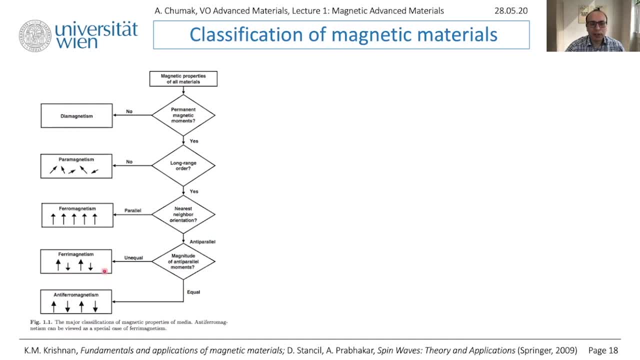 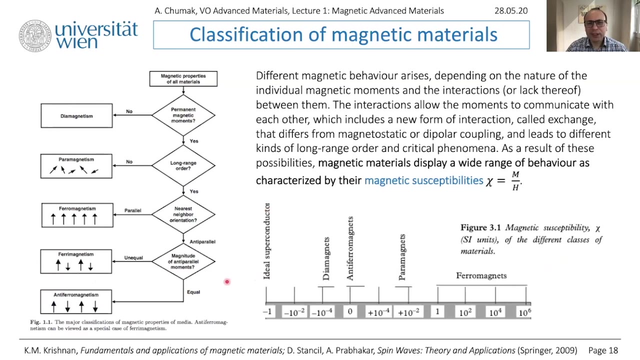 sub-lattice is larger, for example, than this one, then this material is named array magnet. good, so this is the overview of the materials, and now I also would like to show you this picture from Krishnan, because, as I said, if you want to find out what kind of magnetic material you have, first of all you need 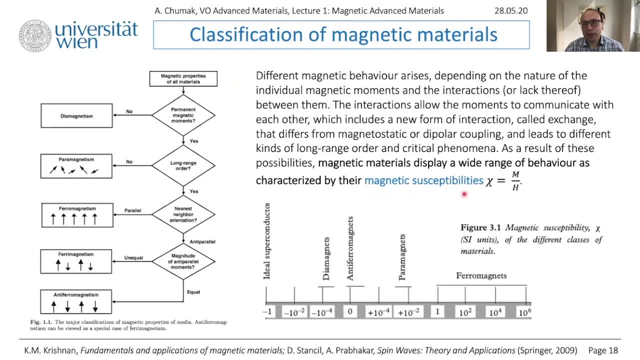 to ask question: what is its magnetic susceptibility? so it gives you the information about response of your body. response means magnetic moment which it will have when you apply some magnetic field age. and here in the left side we are dealing with ideal superconductor and, as we know, when you will put superconductor, 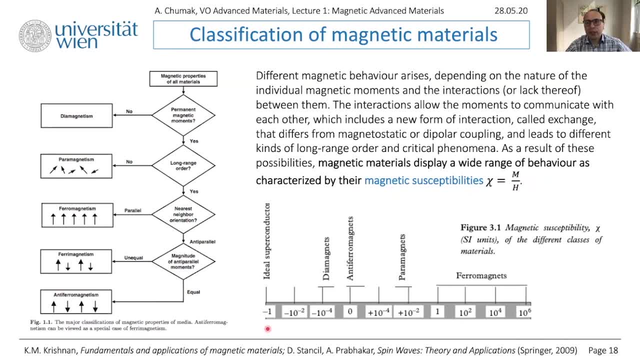 within magnetic field, it will expel the field physically. you can explain it in a way that a superconductor has magnetization which is equal minus applied field age. so m is equal minus age and then immediately from this formula you have the susceptibility of superconductor. 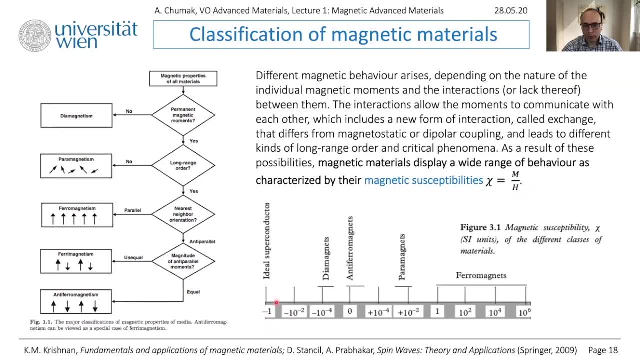 is minus one. good then when we move on we are coming to diamagnets. so diamagnets are, by the way, a superconductor. it's named as an ideal diamagnet and the sense that it's a susceptibility. absolute value of susceptibility is rather large, but 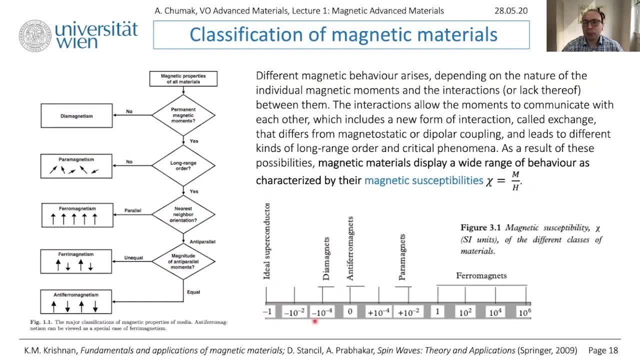 important is that in both cases, susceptibility is negative. it means following the diamagnets. first of all, it's not fully non-magnetic. there is some response of this material to the applied magnetic field and this response is negative, meaning that your magnetic moments will be oriented in the opposite direction to the applied magnetic field. that's why it's. 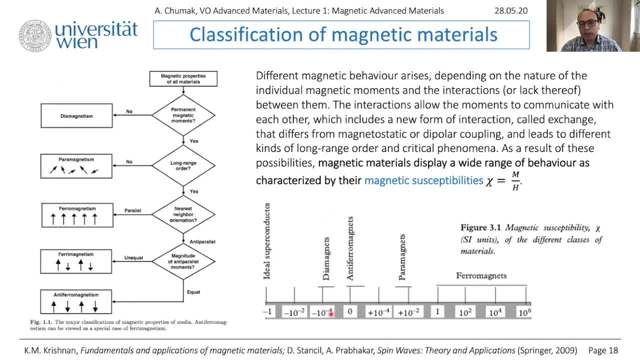 negative. and next what we have to see that? you see, this response is very weak: 10 to the power minus 4. so it means the diamagnets are magnetic but very weak. afterwards we are switching to antiferromagnets and, as we discussed, it's 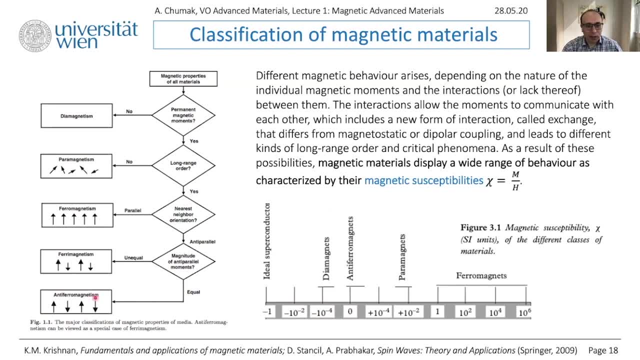 a case when you they are kind of strongly magnetic but you have these two sublattices and magnetic response from one sublattice will be always compensated by the response of the second sublattice. therefore, if you will check macroscopic parameters of antiferromagnet, it looks like completely non-magnetic, unless you will apply. 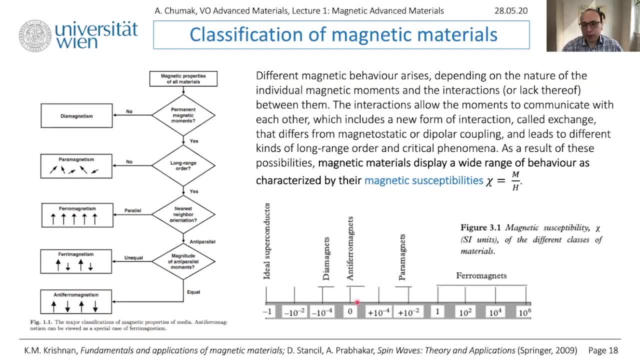 some huge field and but in the simplest case you can say that antiferromagnet has zero susceptibility. so then we switch the sign of our susceptibility. so now we have positive means that if you have some magnetic moments and you apply magnetic field, these magnetic moments will be trying to point in the same direction, like 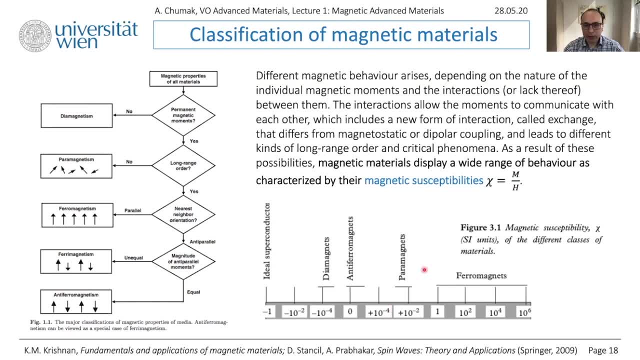 applied field, and here we have paramagnets. so paramagnets have positive chi and the value is not very large. so 10 to the power minus 2, which means that they are not strongly magnetic. at the same time the magnetic response, let's say up to two orders of magnitude more pronounced than for diamagnets. 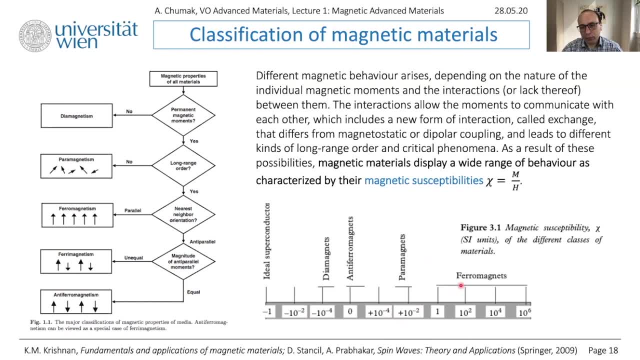 and finally we are coming to ferromagnets. ferromagnets, that's what we, in our everyday life we get used to as simply magnet, and here you see that it's positive. but also its susceptibility can be more than one. more than one means that your magnetic, that your solid body can create. 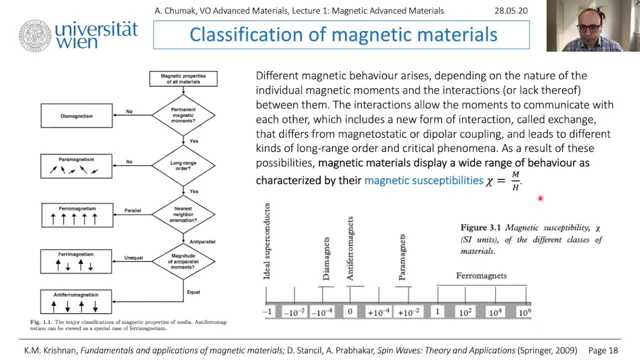 fields on, since on its own that your total field will be larger than applied field h, original. okay, so that's it about the general classification of magnetic materials. now I think we have a very nice overview and are ready to come to each of these types of magnetic materials a bit more in. 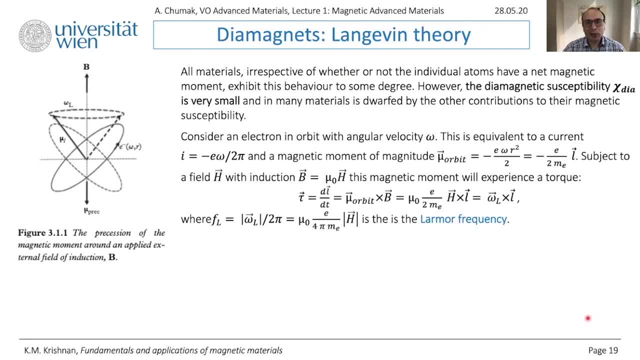 depth, and I would like to start with diamagnets, and here we are talking about so-called longevity theory. first, what we need to keep in mind when we're talking about diamagnets is that, in fact, every atom is diamagnetic or it has some properties of diamagnets. 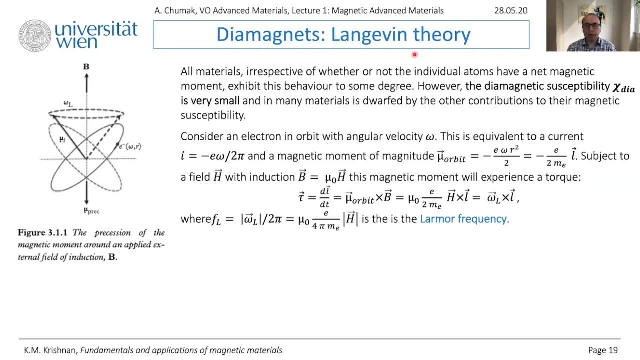 nevertheless, the point is that diamagnetism, this magnetic response, is weak compared to paramagnetism and so on. therefore, in most of the cases, if you have some paramagnetic response or something, you simply do not see diamagnetic contribution to it, and in this case, diamagnetism is simply ignored. nevertheless, you keep in mind that diamagnetic susceptibility. 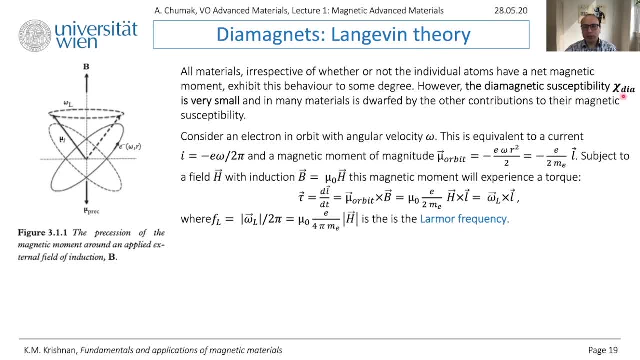 is, in principle, present in every atom, just small, and it can be not visible. so where it comes from? let us have a look first on this orbital. so this is our electron hydrogen model, the warm model of atom which we discussed, and here is a electron which is flying. 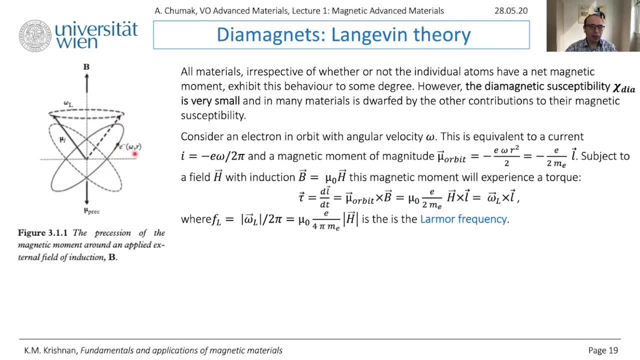 around with some circular frequency, with some radius r and, as we discussed, the motion of this electrons is charged, will create a magnetic moment, orbital magnetic moment, mu l, pointing in this direction so that it will create a current, as we were talking in the previous lectures. and here is the orbital momentum defined previously. 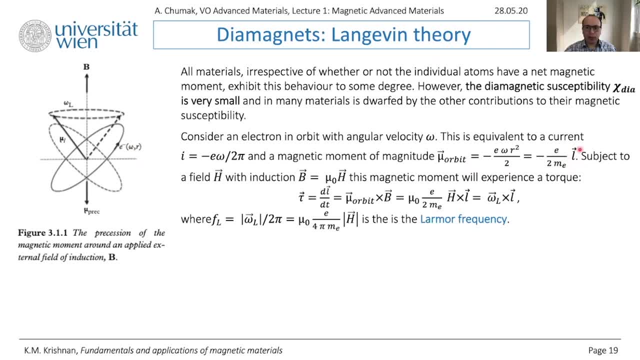 so, and it's coupled also to the angular momentum of the orbital motion of electron. so, and the question now is: what happens if you put this magnetic moment into external field? each, as we know already, this magnetic moment will experience a torque tau, which can be found simply as a cross product of 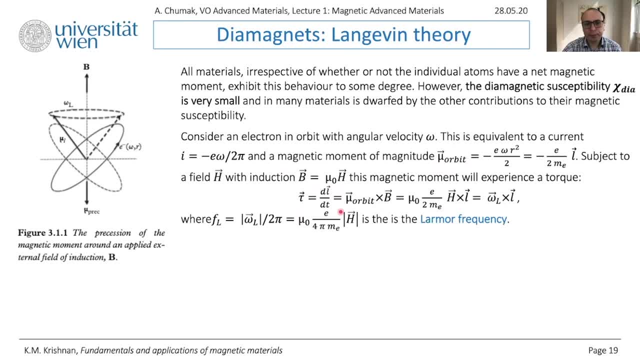 magnetic moment with a magnetic inductance B. by definition, torque also is a very temporal evolution of orbital momentum, and for us it's important that now, instead of this orbital momentum, we can simply plug in this formula, and instead of inductance B we plug in mu, zero, H, more. 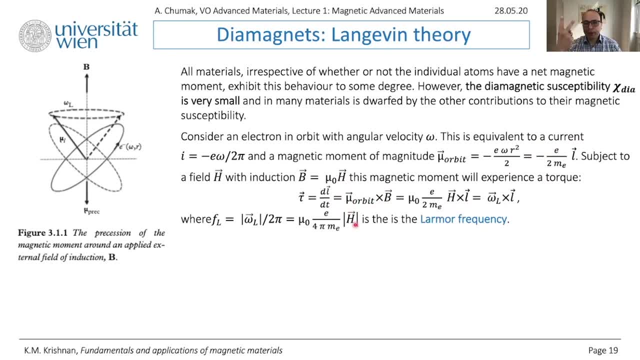 over. you see, I have replaced them. I changed exchange mu and b with places. therefore, we have no minus here, and this is done especially in order to be able to get this new parameter, omega l, which is a vector. so, this is a vector. nevertheless, if you will take its absolute value and if you will divide it with 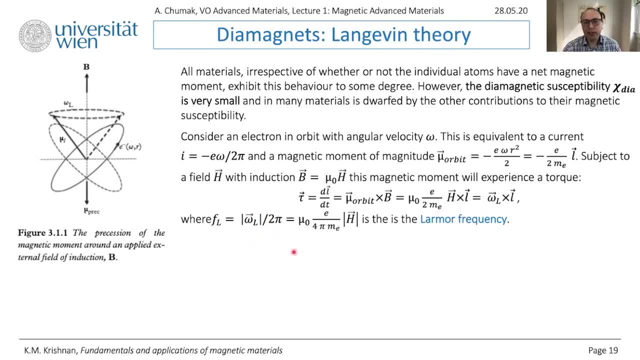 2 pi in order to switch from circular frequency to linear frequency, then this is nothing else as known to you: larmor frequency. so it means that this physics describes simply a larmor precession. when you have magnetic moment of atom, you put it inside magnetic field, it will start to process. 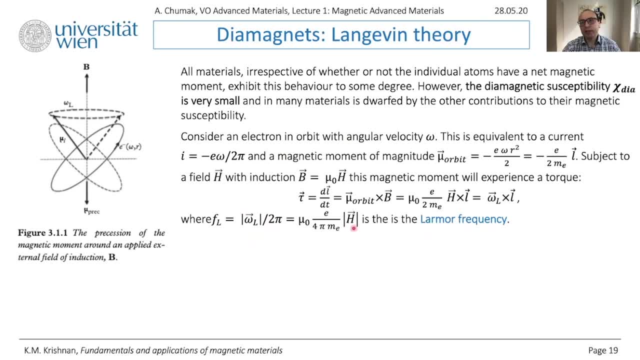 a frequency of precession is proportional to the applied magnetic field. h. the next question you have to ask what happens now, how this precession influences the magnetic response of our material. and this is very easy because this precession will induce a new magnetic moment which can be found like that. you can check all the steps in krishna, how it's derived. 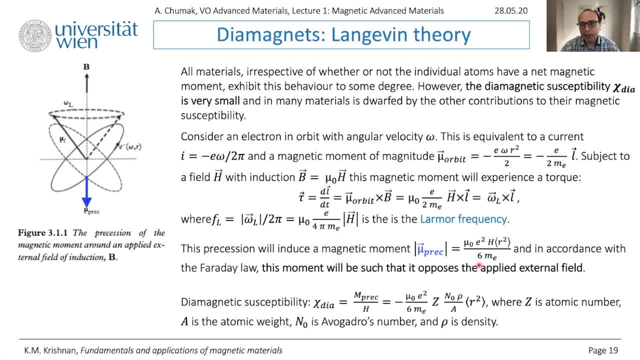 here i just briefly explain you the main idea. and idea is that this formula is very similar to that one. you see, like we originally obtained the simplest orbital magnetic moment of electron. now, instead of omega here i put new omega, larmor precession, this value. so now we are talking about new frequency. 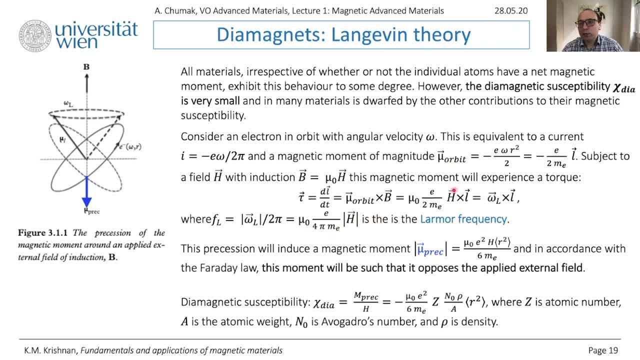 a new, new circular frequency and of course we do not have any more uh, this, uh, atomic orbital r, but we need to have a new value. but doing some summarization, so first of all we need to understand that if you will consider now this precession, it creates a new loop. 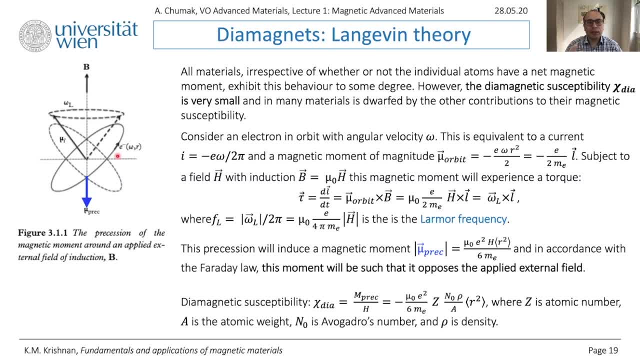 of any of this current and the diameter, the radius of this loop is not stable, so it will be changing in time the process of precession. nevertheless, you still can couple its average ratio. you see, this means, as we are talking about r squared averaged, you see the variation that is. 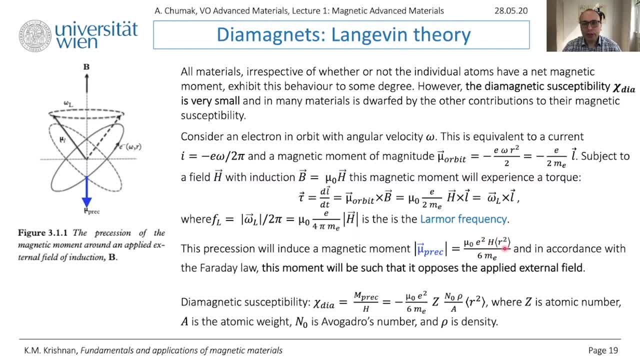 we are talking about r squared averaged. you see the variation. r squared average you can couple to the original radius of precession of your electron, but you need here an additional factor of three. That's why the magnetic moment created by the Lermont precession 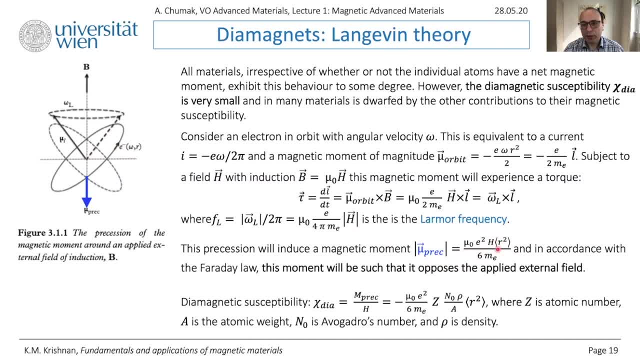 can be found in such form where you have average R-square and divided over 6 Me and is proportional to applied field H, because it creates a magnetic moment. And here it's a formula for the absolute value of new magnetic moment created by the Lermont precession. 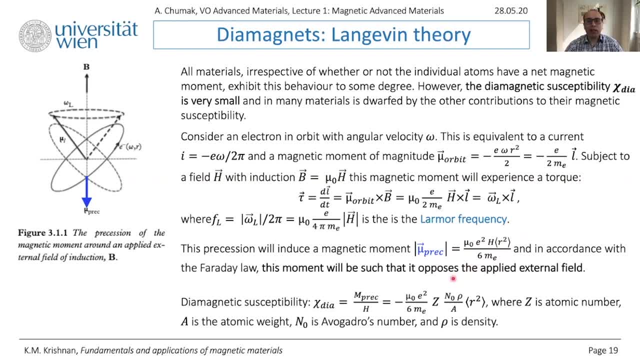 And the question is where it points. And here it's easy, because, according to the Faraday law, the new magnetic moment which will be created by your atom will be pointed in such direction in order to compensate- actually compensate- the applied magnetic field. So it means, if you 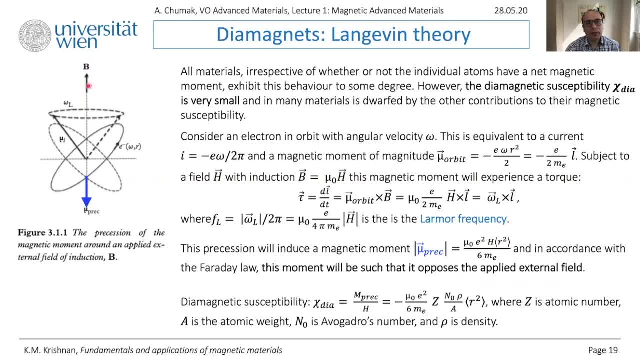 magnetic inductance is pointing up, like it's shown in this figure. the new magnetic moment associated with the Lermont precession will be pointing in the opposite direction, like it's shown here, And this is a reason why the magnetic susceptibility of diamagnet is negative. 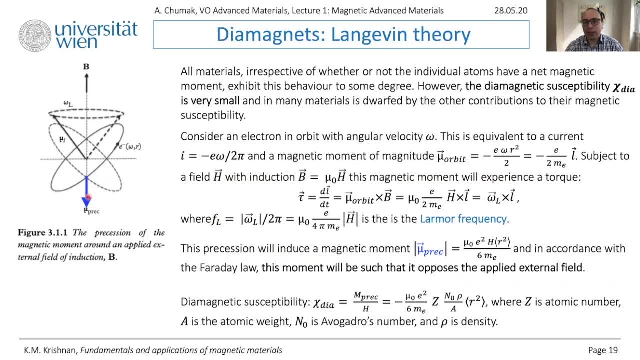 because mu is trying to point in the opposite direction to that magnetic field. Then what we can do, having this magnetic moment for each atom, we can now calculate the diamagnetic susceptibility. In order to do so, you need first of all to find magnetization m. 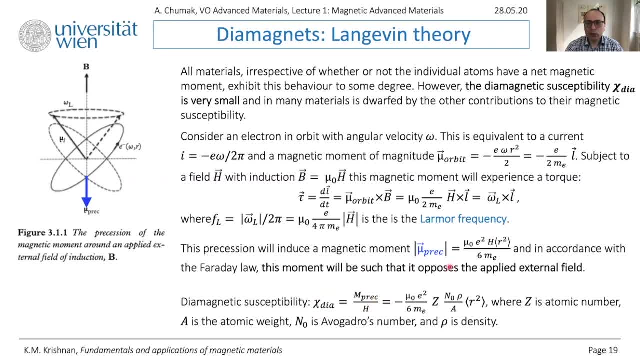 and magnetization. you just need to summarize more or less all magnetic moments you have in your system, And that's why in this formula we see appearance of such parameters as atomic number, so how many electrons you have in your system. And also magnetization: is total magnetic moment per volume? 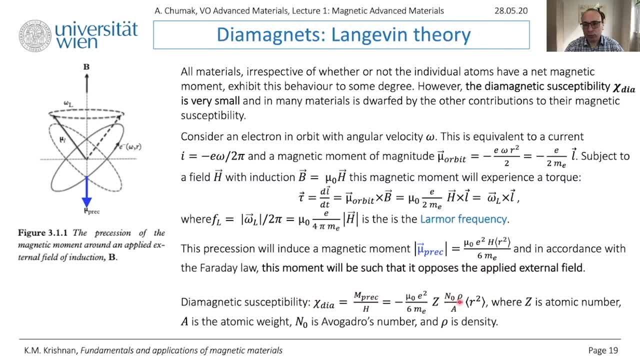 Therefore we need also these two parameters, which is rho is a density and m0 is an Avogadro number, And H simply disappears because susceptibility is total magnetic moment divided by H. Therefore H disappears and here is your value for diamagnetic susceptibility. 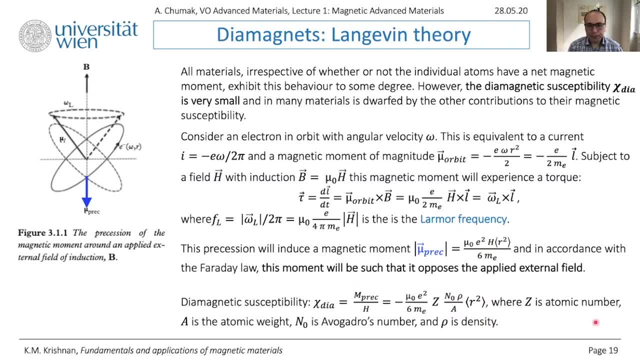 Good To summarize a few comments. First of all, usually people think about diamagnetic materials like about non-magnetic materials. It's not, strictly speaking, it's not correct, because we clearly see here that there is magnetic response of diamagnet to the applied magnetic field. 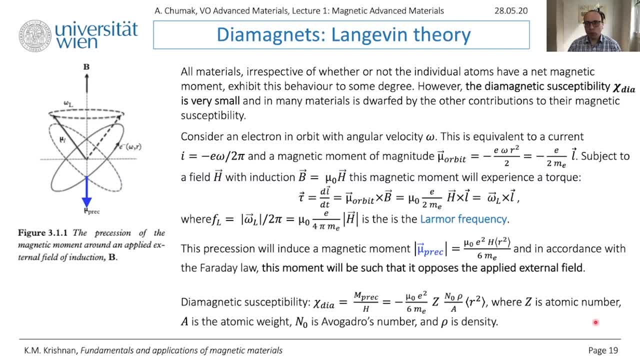 Nevertheless, we keep in mind that this response is much smaller than other magnetic responses which you can have in the system. But second, what you need to keep in mind is that this magnetic moment appears only after you applied magnetic field. So diamagnet is really absolutely non-magnetic as soon as you have no applied magnetic field. 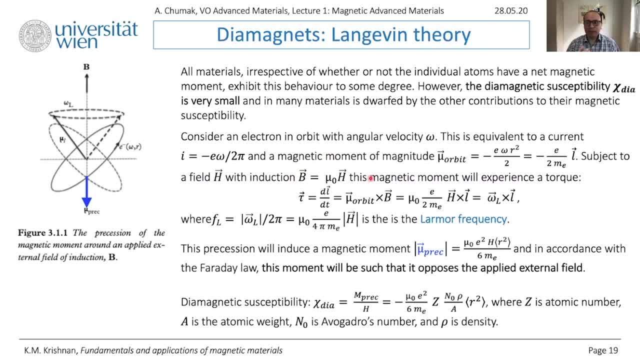 But if you have field, the application of the field creates this magnetic moment And this magnetic moment is pointing in the opposite direction, trying to minimize it. That's why we have creation of magnetic moment. with application of magnetic field, This magnetic moment is small and it's pointing in the direction opposite to the applied magnetic field. 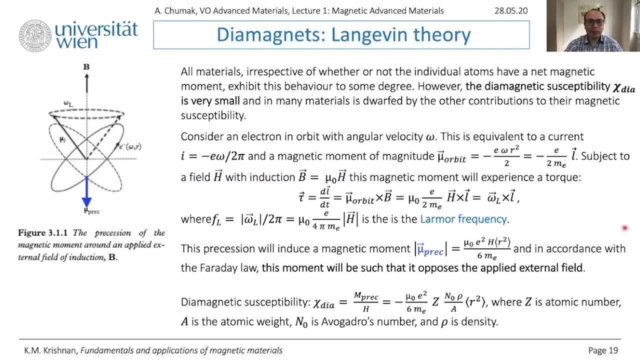 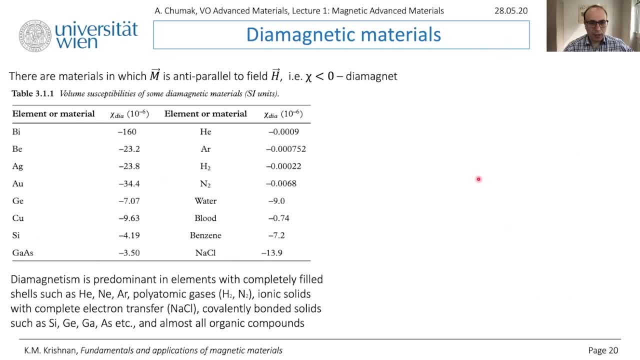 So these are the basics about diamagnets, And let us have a look which materials can be diamagnetic. Principally, of course, as I said, we want to avoid any uncompensated spin, For example, of electrons, something like this: 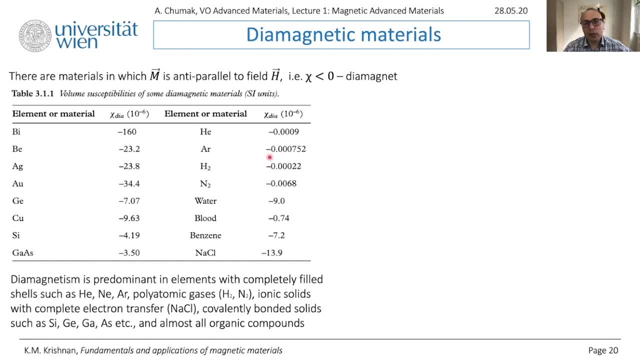 Therefore, first of all, we need to consider noble gases like argon, for example, where all electron shells are fully filled. In this case, it means that orbital momentum is compensated and spin, So it means that you always have two spins pointing in opposite direction. 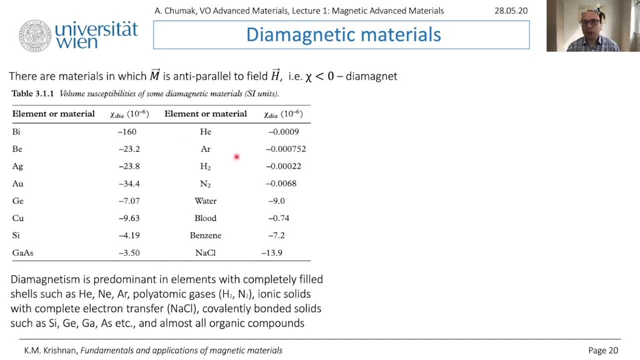 which compensate each other. So it's very like neutral atoms and also neutral sense of magnetic response And in this case you can feel, you can see this small diamagnetic response of your atom. That's why these gases are diamagnetic. Many metals, silver, gold- they are also diamagnetic. 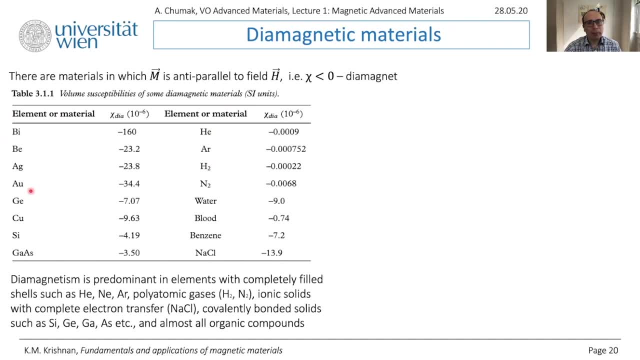 But here we need to be careful, because to describe diamagnetism, to describe magnetic response of metals, you need different models, You need to operate with energy bands, And then some materials are diamagnetic, some are paramagnetic And it's a bit more complicated to explain that. 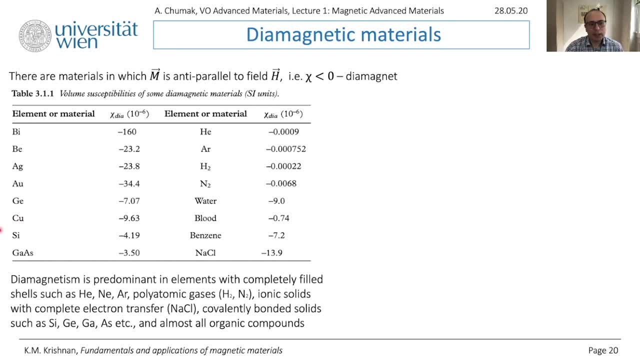 But just keep in mind that also copper is diamagnetic. Then we have semiconductors: silicon, gallium, arsenide, They are diamagnetic molecules H2, N2 are diamagnetic. And then also very interesting, that water and our blood. 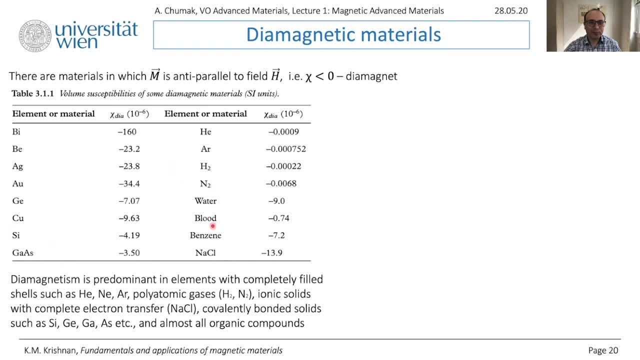 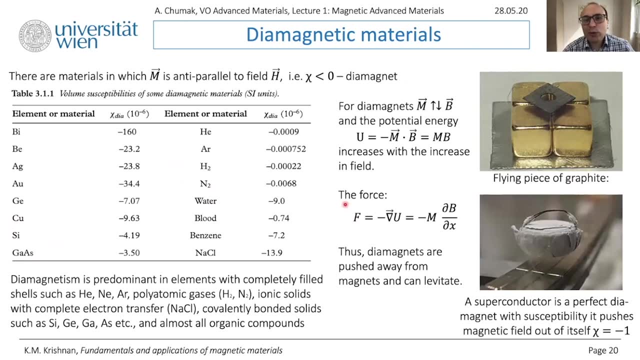 so human being is also a diamagnet. What kind of interesting experiment, people, you can do with diamagnet, And one of them is levitation. So since susceptibility for diamagnet is negative, high is negative, then magnetic moment magnetization will be pointing in the opposite direction. 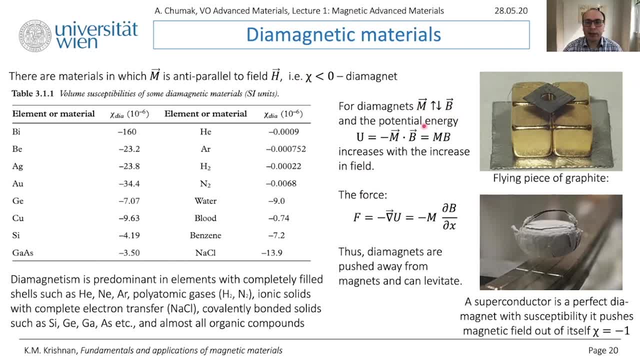 to the black magnetic field. But, as we have seen, the potential energy of a magnetic moment placed within the magnetic field, it can be found as a scalar product with minus, And now, since you have here minus M, it's proportional to MB. 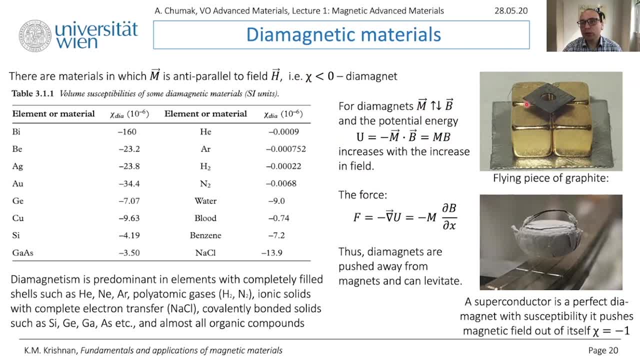 It means that if you take your diamagnet and put it closer to your permanent magnet, namely increasing field magnetic inductance B, it means that you increase your potential energy And system tries of course to minimize the potential energy. But in this case what happens? that your diamagnet is pushed away. 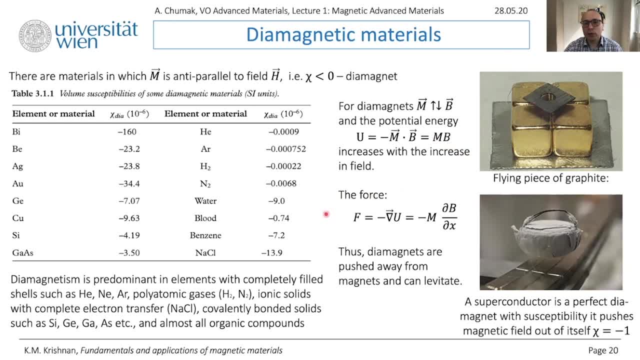 from certain magnetic field Or, if you want, you can find a force as a gradient of this potential energy, And if you consider only one direction, then you can get such a force, a formula, And in this concrete configuration it means that you will get some balance. 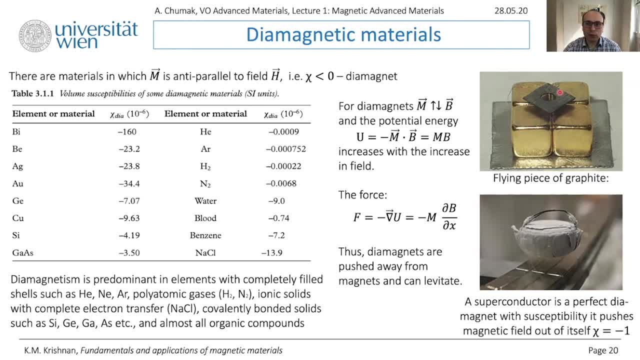 between gravitational force, Mg, which tries to put your piece of graphite, in this case, down, and force created by the magnet which is pulling it up, And this experiment you can easily perform, Or there are other many experiments. You can find many different nice YouTube videos about superconductors. 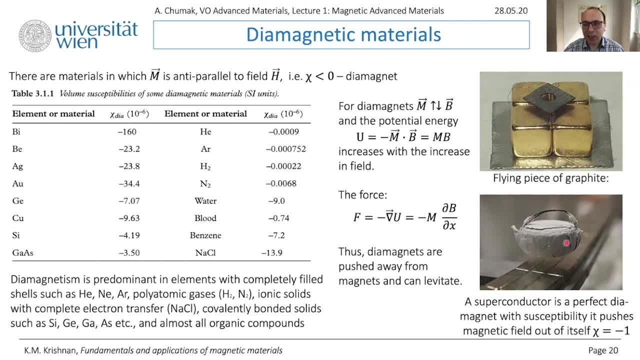 So if this is a superconductor, which is an ideal diamagnet and these are just some permanent magnets, it will be levitating. And, by the way, there is this fast train, I think, in Shanghai airport, which is really the whole levitating train. 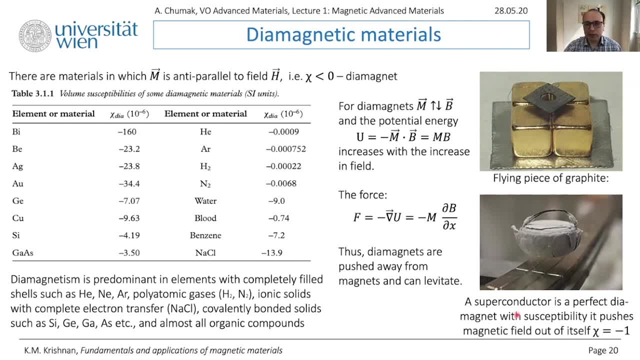 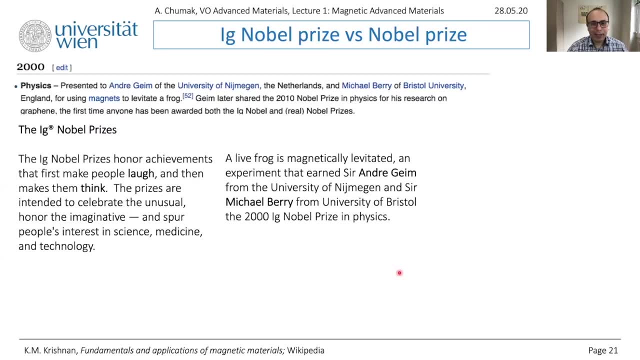 which can go very fast, And this is particularly the physical principle why it works. And now I would like to take a minute of break and just present you a brief story about the Ig Nobel Prize. All of you know Nobel Prize, which is given for serious scientific achievements. 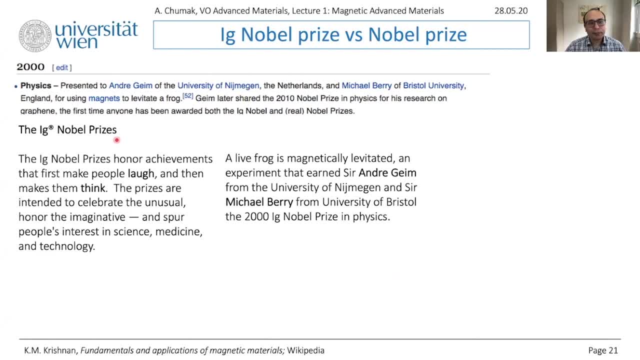 in different fields of science, And there is a so-called anti-Nobel Prize, Ig Nobel Prize, which is given for some strange and kind of useless achievement, And the philosophy, of course, is very good, but there is a lot behind that. we need to laugh in order to think. 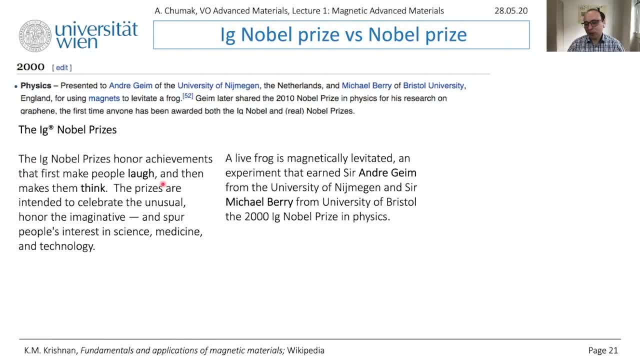 So it's just a process which not only makes our life more interesting, but also it stimulates the way of thinking. And as a good proof for this is a story with Dr Andre Geim, who got an Ig Nobel Prize in 2000. 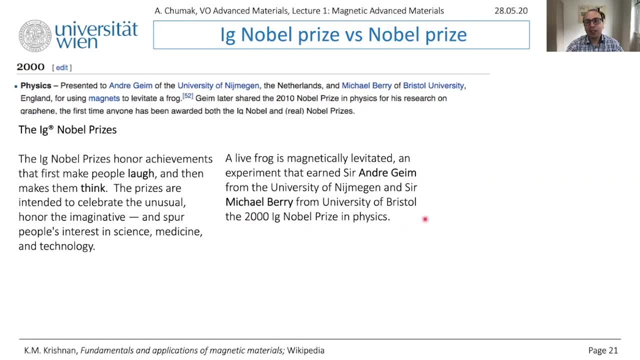 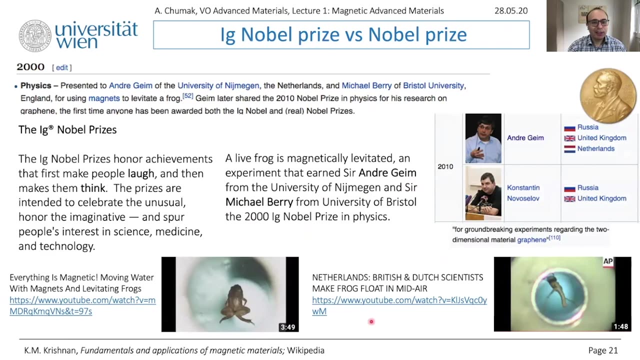 for levitating frog, which you will see in a minute. Ten years later he got a real Nobel Prize for the discovery of graphene. So it's a nice story And here is the movie I would like to show you. But before 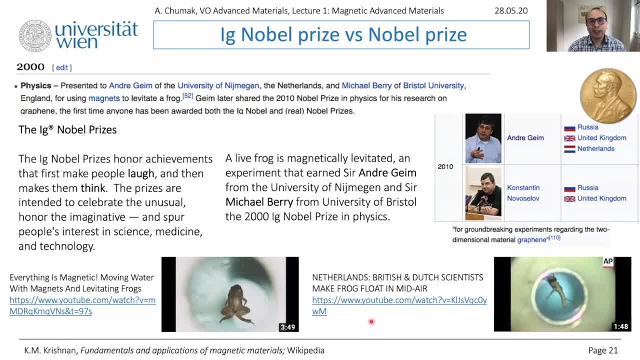 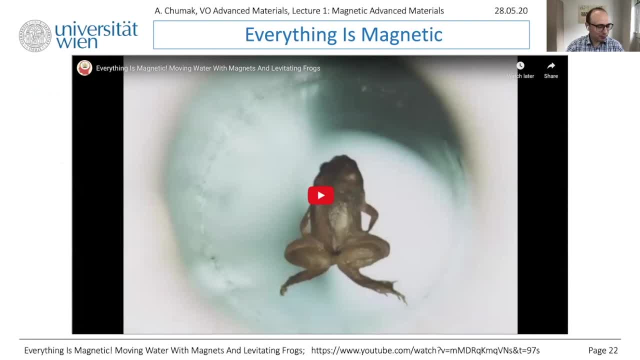 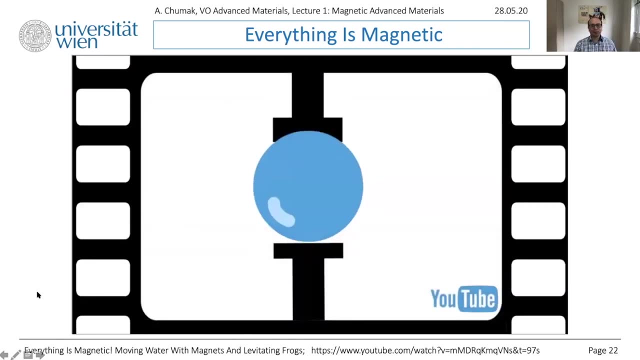 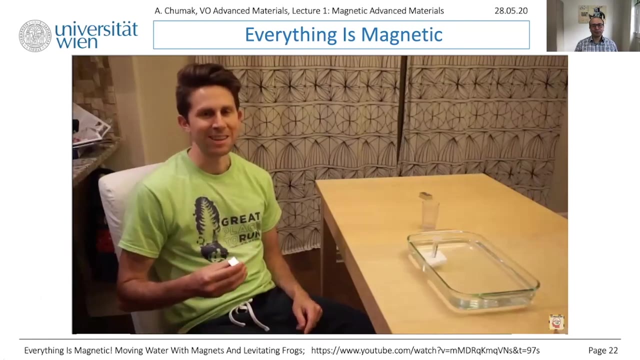 I want to show you briefly another movie which shows that we are really surrounded by diamagnetic materials. Okay, let us have a look at the movie. Okay, hey, everybody, Today I'm going to show you how everything is magnetic. So I have my super strong neodymium magnet. 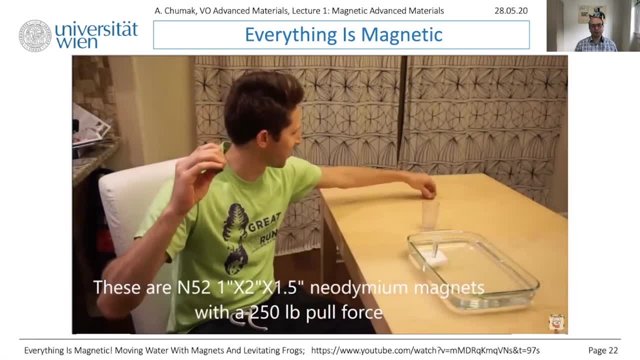 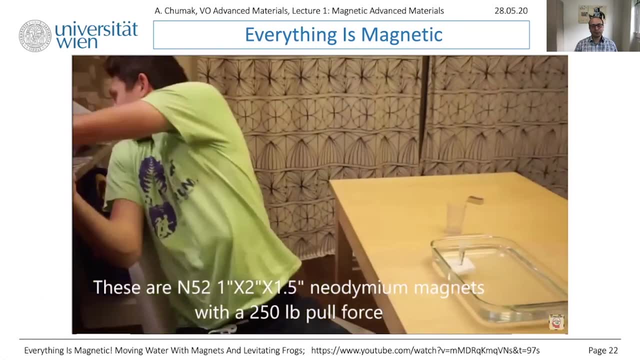 These magnets will crush your fingers. They are very strong. I have two of them, Notice I have this one clear over here. So I just typically keep them in my kitchen mitts because if they get stuck together, they're not coming apart again. 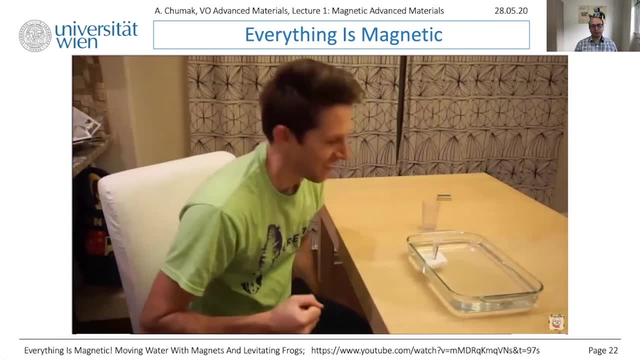 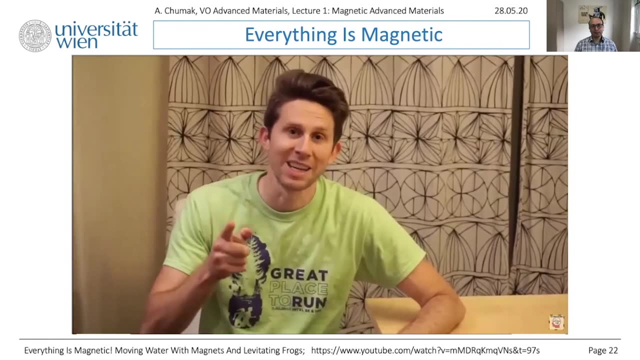 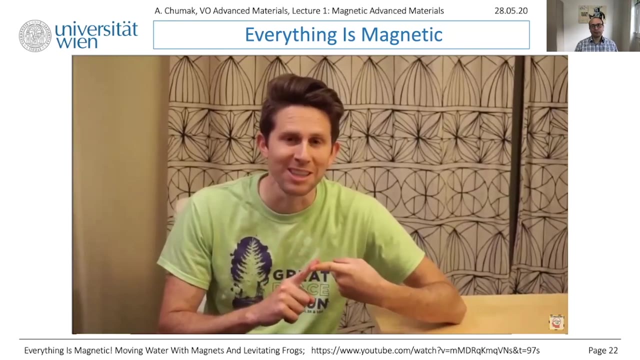 So what I'm going to show you today is how everything is magnetic. So we all know that, yes, a magnet can attract another magnet, But what you might not have known is that everything is magnetic: Water, air, people, wood. So I'll show you these effects. 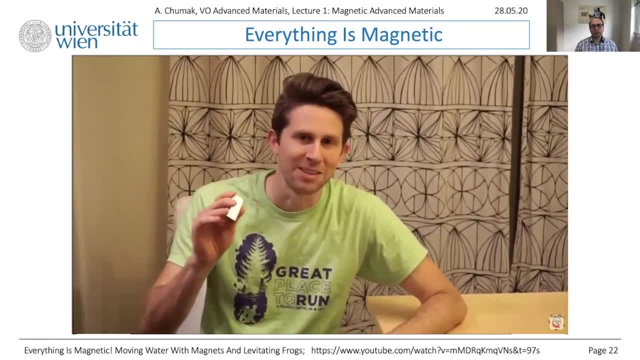 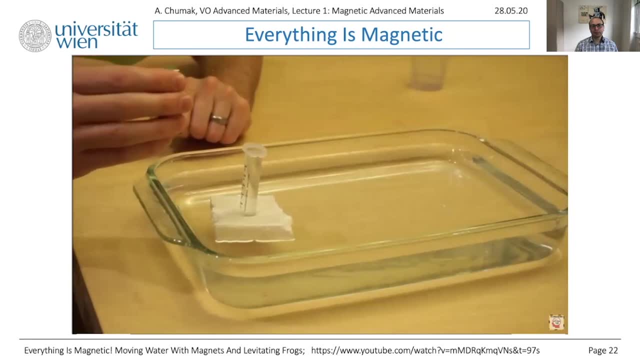 of diamagnetism. Everything repels a magnet. I'll show you that. What I have here is a syringe full of water, and I have my strong magnet. I'm not going to touch the magnet too, I'm just going to bring it close. 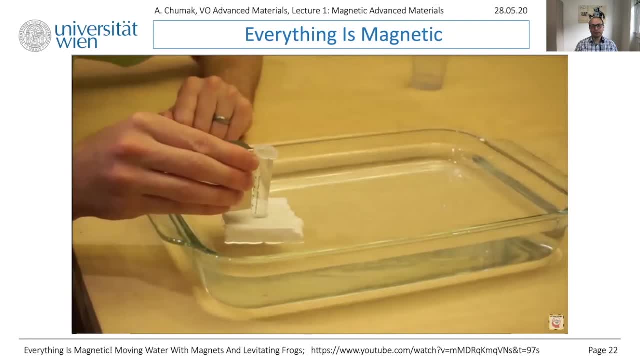 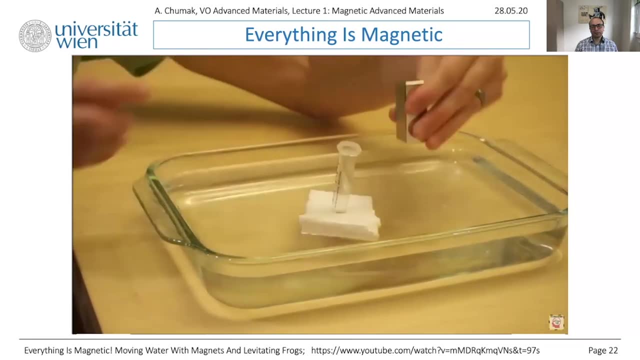 and the water is going to repel the magnet and get pushed. It kind of looks like you're touching it. I'm not touching it. Prove it. Oh, there you go, Let's push it back. I'm not touching it. 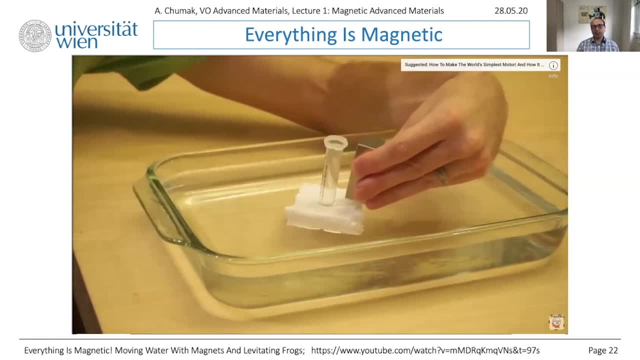 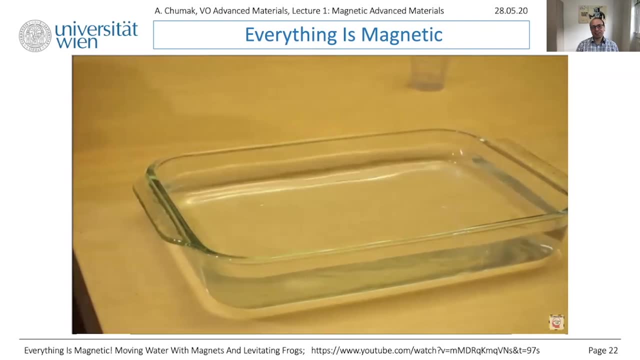 So we can clearly see that water is diamagnetic. So water repels a magnet. Another thing that repels a magnet is wood. So here's an ordinary block of wood. I'm going to bring the magnet close to it, but not touch it. 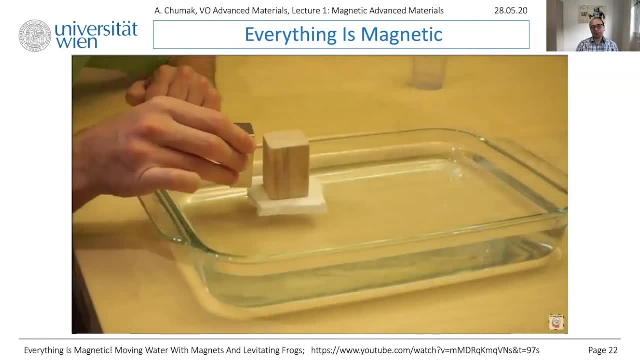 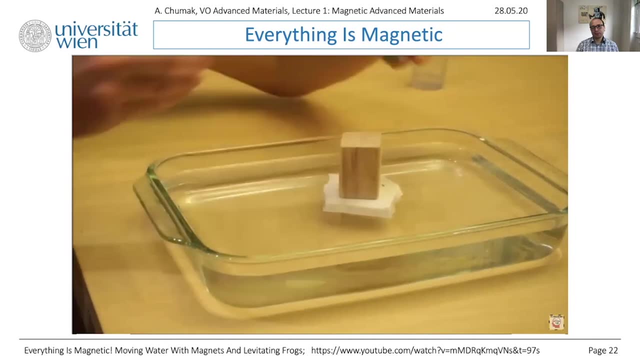 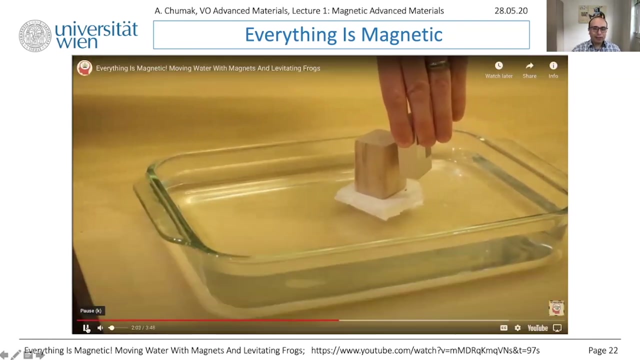 Let's change that angle. Okay, See how it's not touching it, pushing it away. I can't really see It's stopping it. Let's push it away. So how is it doing this? So diamagnetism is a quantum mechanical effect. 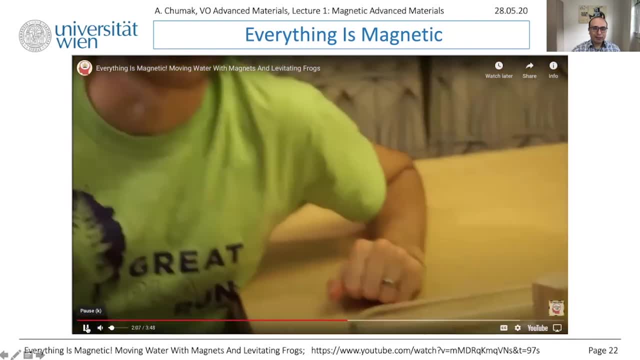 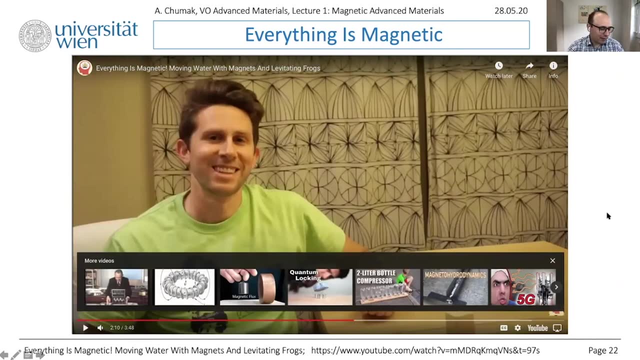 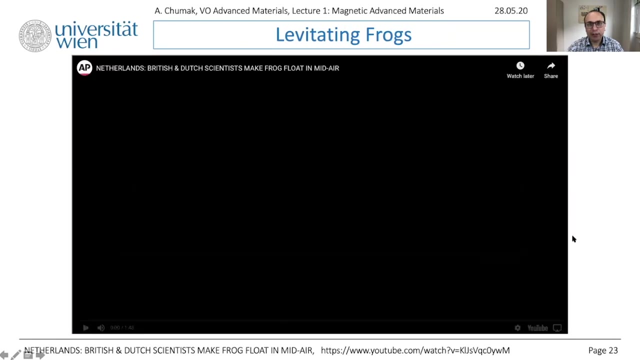 which I won't get into, but essentially it's repelling the magnetic field. So principally we can move on. You have seen the experiments and you got already the understanding why it's diamagnetic and why it is pushed away from a light magnetic field. 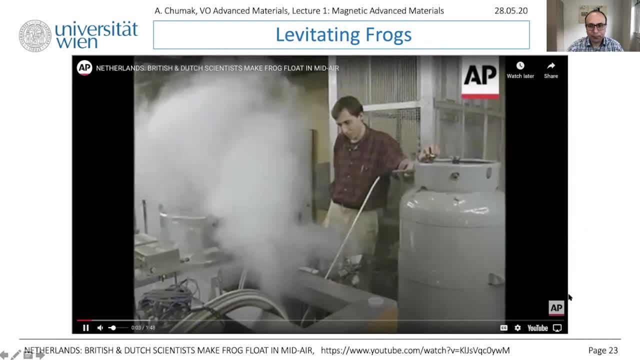 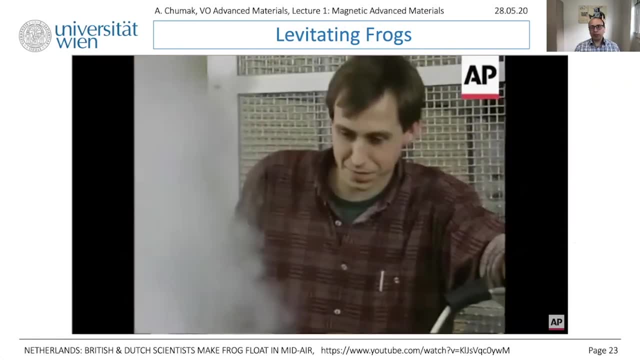 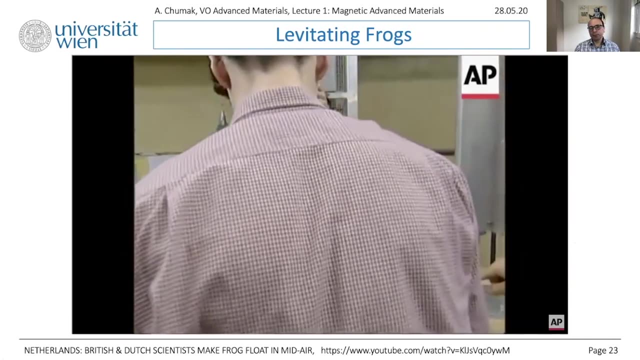 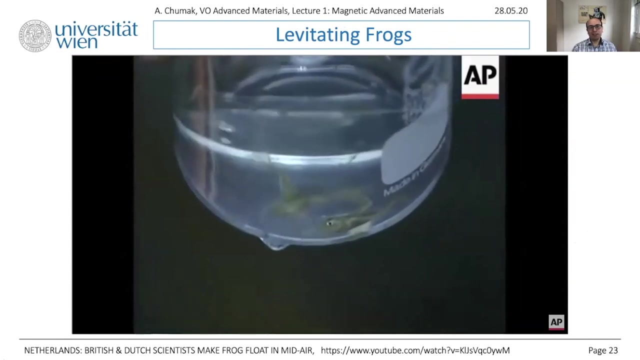 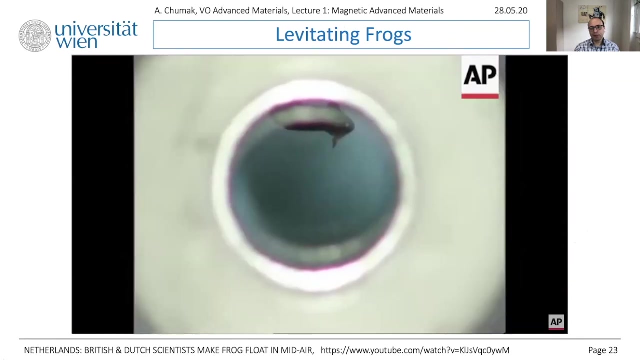 And I'm switching to the next experiment. In order to perform this experiment, you need superconducting magnets in order to create a huge or a large magnetic field. That's why you've seen liquid nitrogen, And this is this little frog, And now camera is showing you the 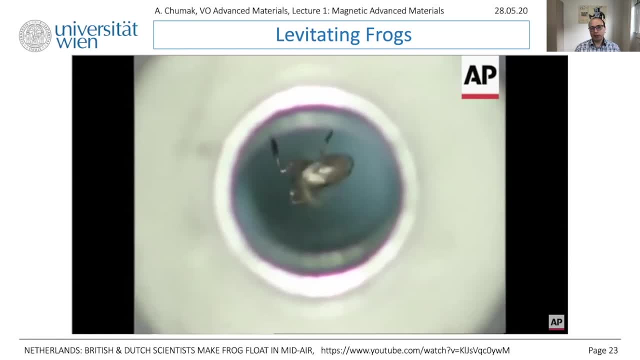 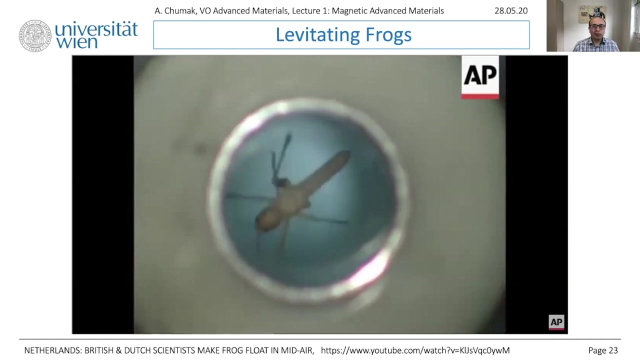 magnet And you can see that frog is levitating. It's alive. It doesn't feel any hurt or something, Maybe a little discomfort, But it's a nice experiment which proves that alive beings are diamagnetic. So if you will find a way to create, 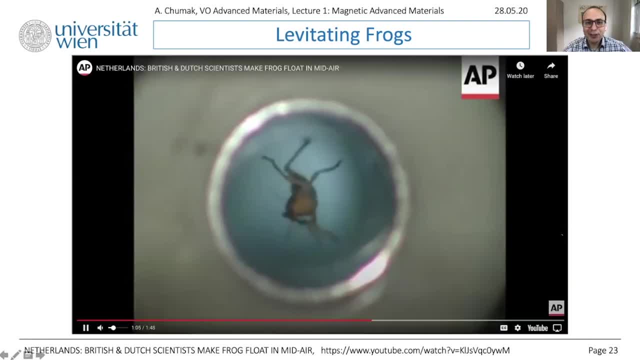 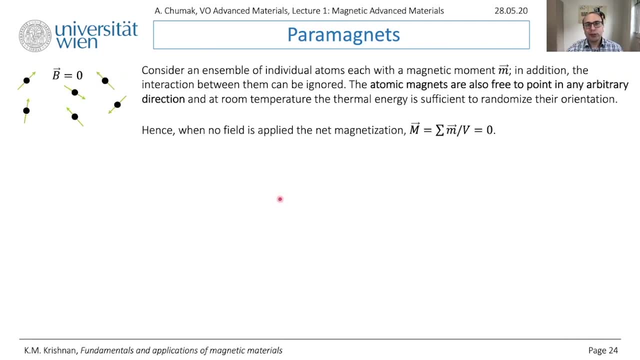 larger, not magnetic field. you can also levitate As a frog. And now I would like to switch to paramagnets, As opposite to diamagnets, paramagnet is a material in which magnetic moments are present all the time, even if you have no applied magnetic field. 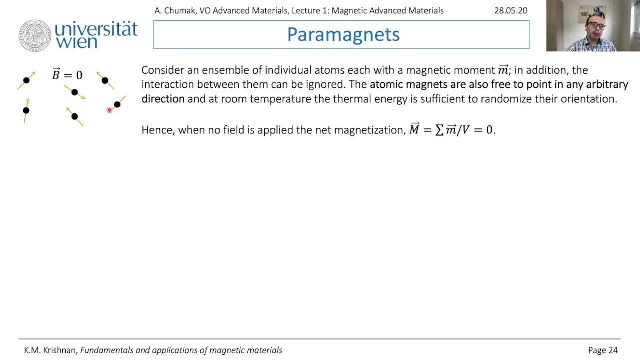 Usually these magnetic moments are depicted with such arrows And in the case of absent magnetic field they usually point in all possible directions. So they are independent and temperature KBT brings a chaos into the system and they simply change their orientation all possible way. That's why all possible directions. 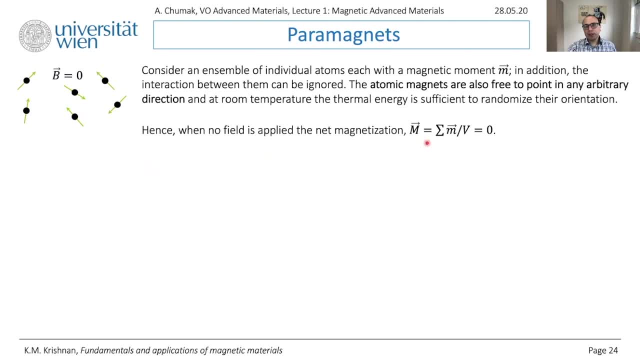 That is why, when you will try to find magnetization of paramagnetic material and you summarize magnetic moments for all possible magnetic, You will try to find macroscopic response, Magnetic response from all magnetic moments. So this is your magnetization, It's vector, sum of all. 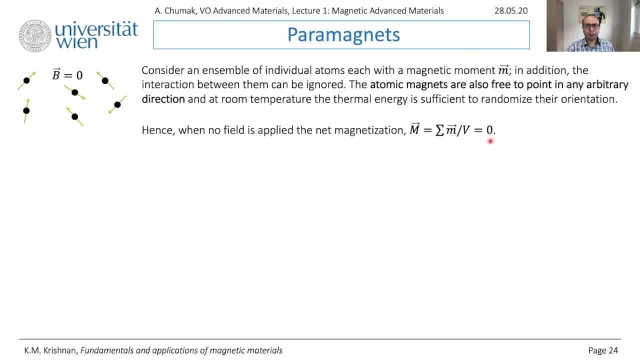 magnetic moments divided with the volume of your body, You will get zero here. So it means that for each magnetic moment you just point in one direction, There will be another one pointing in the opposite direction, which compensates its response. Next question is: what happens? 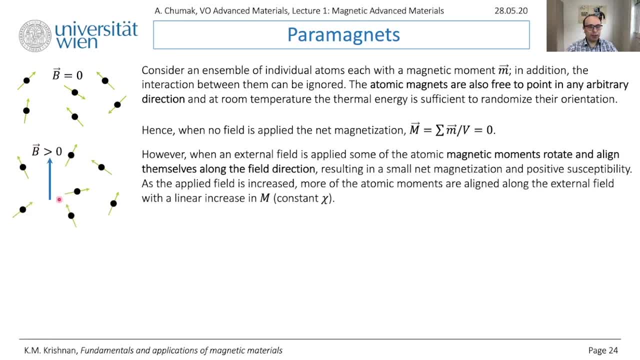 if we apply some magnetic field, You see that usually in this case you still have chaos. But if you will look more carefully, you see that now more arrows are tending to point along the applied field and less arrows are pointing in the opposite direction. 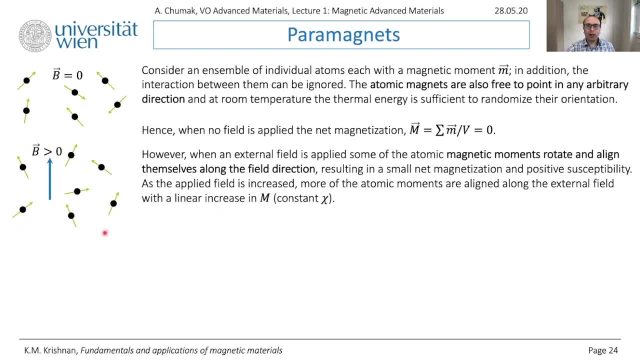 So it means that you still have this chaos, but already some visibility of order shows up here, Since most of them say tried to point more along this direction and, as a result, your magnetization- in this case the total magnetic moment, will not be zero anymore. 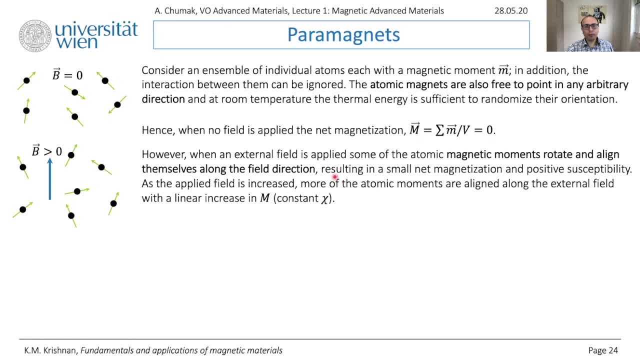 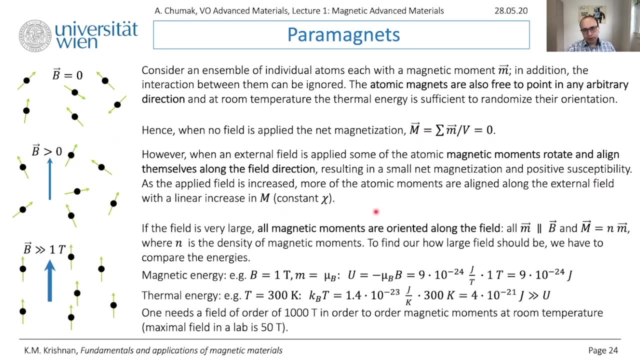 It will be small but not zero, And M will be pointing along the applied magnetic field. Therefore we can speak about positive magnetic susceptibility In principle. theoretically, you can reach a third condition if you will apply a huge magnetic field. So one tesla is a field. 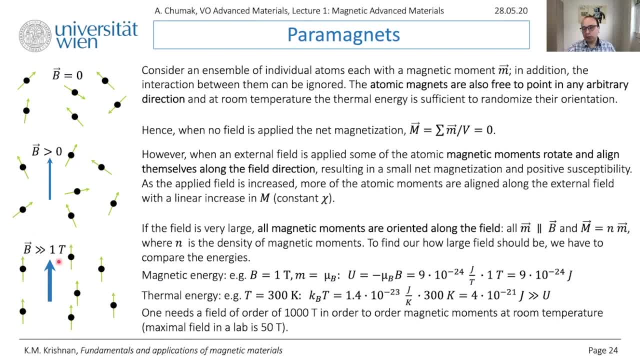 created on a surface, for example, by this neodymium magnet shown by the guy in the video, Or maybe, but you probably would need a bit larger magnet for that. And let us check what should be the field that we can orient all magnetic moments along. 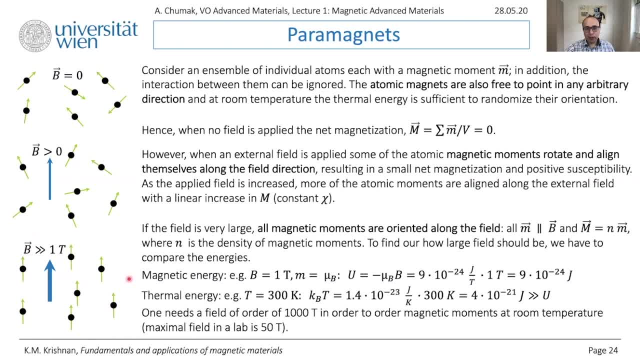 to have fully saturated state at room temperature. For this we need to compare two energies. First of all, magnetic energy. and let us have a look. what will be magnetic energy for this rather large one, tesla field? For magnetic moment, we simply take a magneton bore. 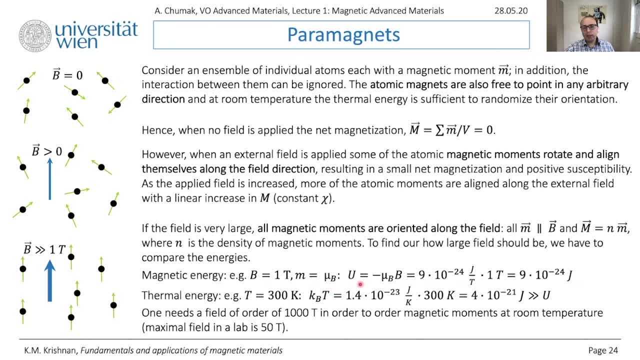 for simplicity, and then our energy. we can make the simplest calculation, which will be nine ten to the power minus twenty four joule. Let us compare it to the thermal energy. Thermal energy is easy, so we are speaking about room temperature, three hundred Kelvin KBT. 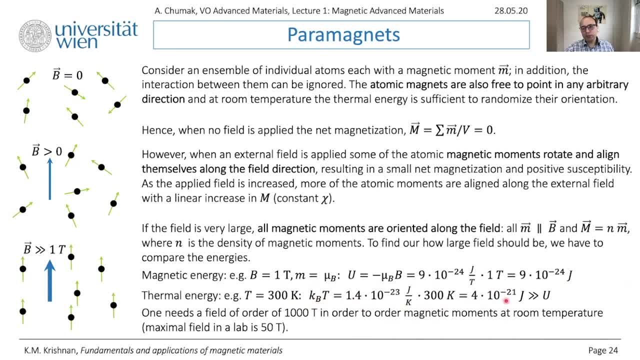 We will get the value four ten minus twenty one joule, which is around three orders of magnitude larger than magnetic energy. So it means even applying such a large field, you will not get magnetic order as it is shown in this picture. If you want to get, 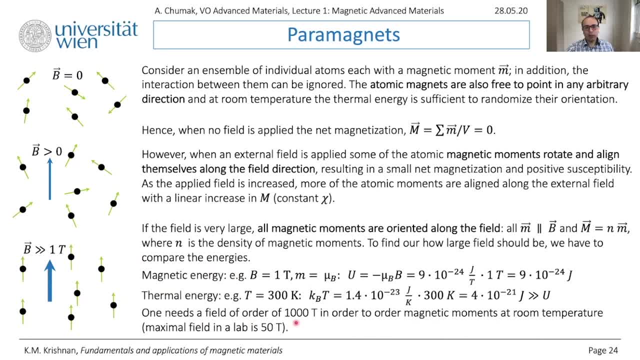 order in the system, one needs to apply fields of order of one thousand tesla which, at least in static regime, is not possible to achieve, to the best of my knowledge At least, in labs, usually people work with fields smaller than fifty tesla, And of course you can. 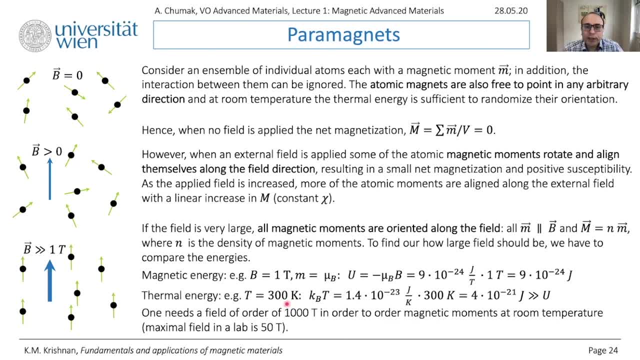 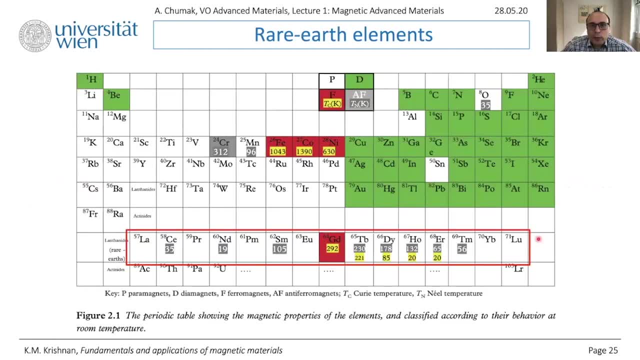 decrease temperature and then you can get saturated state for paramagnets, but it is hard to do it for room temperature. Okay, and now I would like to make a little detour and to focus on lanthanides, metal. So this is periodic table of elements. 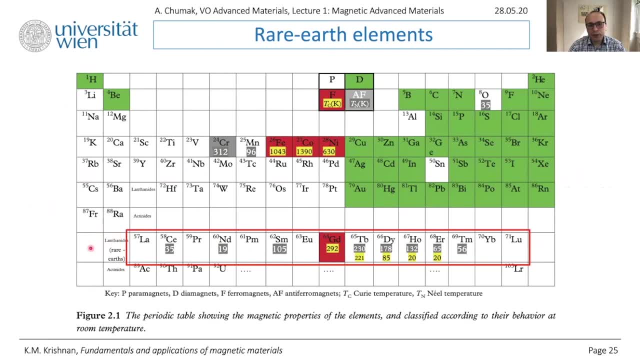 and lanthanides are shown here, and these are materials and you see that some of them are paramagnetic, some of them show anti-paramagnetic behavior at very low temperature, and gadolinium can show also paramagnetic behavior, But usually so you can. for example, 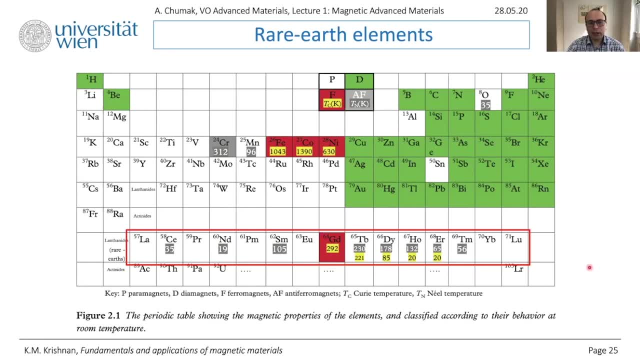 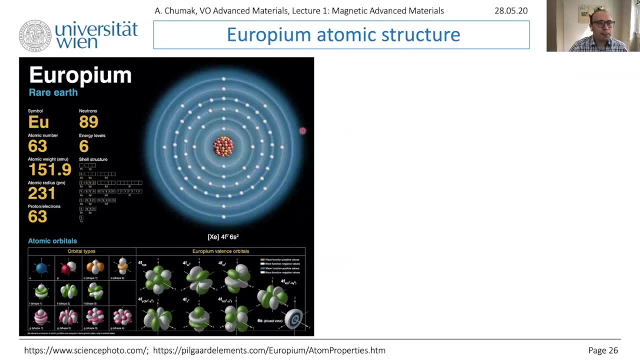 europium. it will be paramagnetic and let us have a look closer to it. First of all, we need to look to have a look at the atomic structure of europium. So it is an element with atomic number 63. that means it has 63. 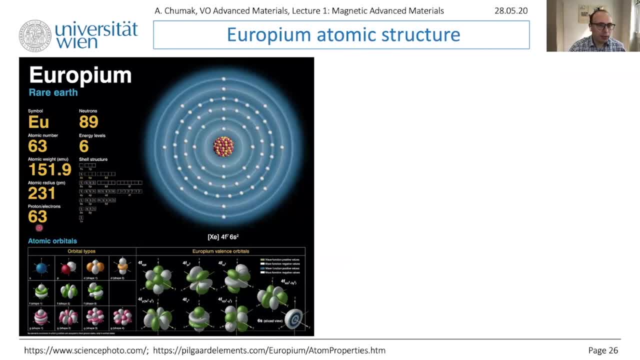 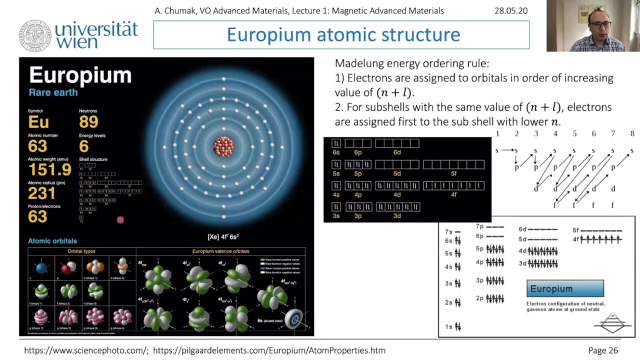 protons nuclear and 63 electrons. Its atomic weight is around 152. that means that in addition you have 89 neutrons in its nuclear And in this picture you see the shell structure and electronic configuration of the atoms. so we are coming in a minute. 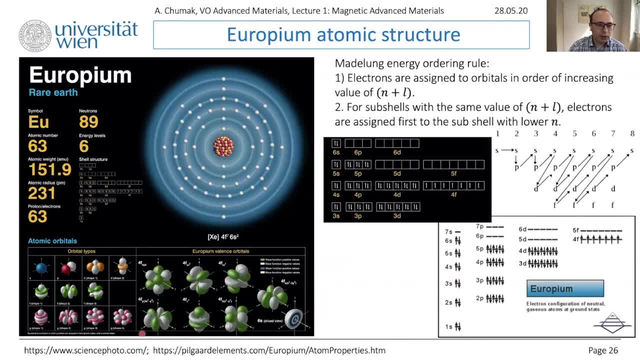 to this, and also here are some pictures of different SPD shells, how they are looking. Okay, and the first question you want to ask is: okay, I have so many energetical levels given by principal quantum number n defined, and how do I fill them? And if you? 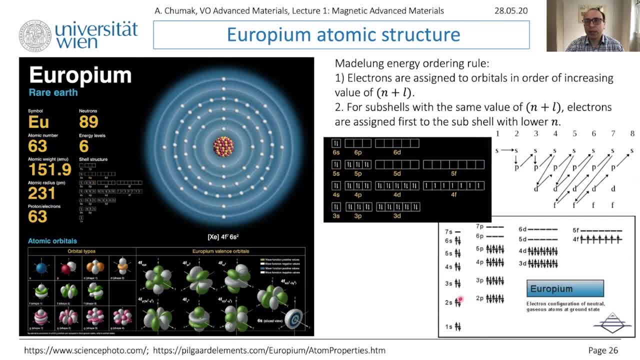 go to the inner shells and so on, but starting from some point, you will not be able to fill simply fully one shell and then switch to next principal quantum number. my system is getting more complicated, and here you're talking about so-called modeling or energy ordering rule. 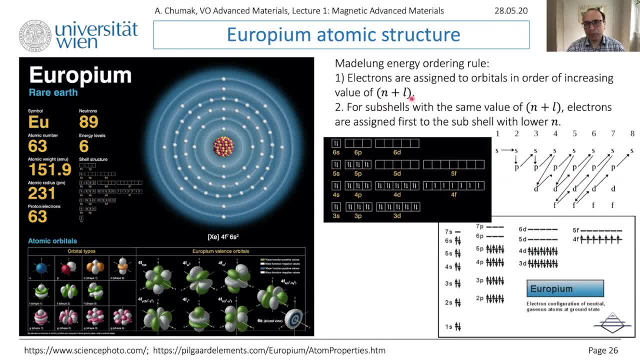 which tells us that electrons are assigned to orbitals in order of increasing value of n plus l and so on. So you need to first fill the shell with two s, two p, three s, three p. then, instead of going to 3d, you are. 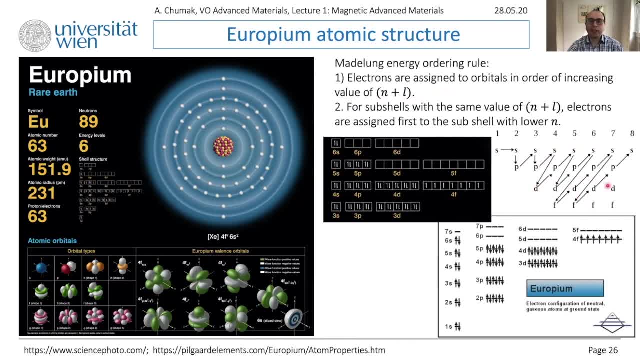 going to 4s and jumping back to 3d, and then the shells are filled in such a way, And that's exactly what you see when energy increases, but then you have after 3p, you have 4s, energy and then 3d. 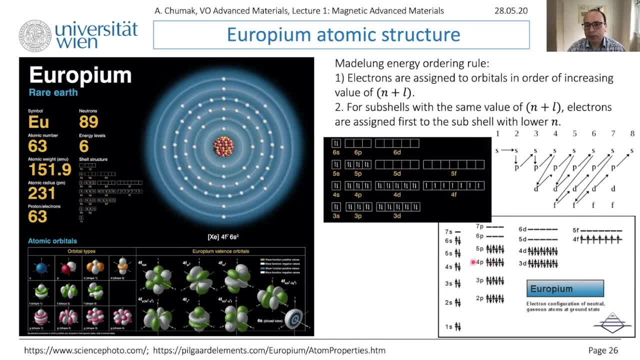 energy, because on afterwards, this level will be filled, then 4p, then you're jumping to 5s, 5p then coming back to 4d. therefore, it's a question how you need just keep in mind that when we are talking about properties of 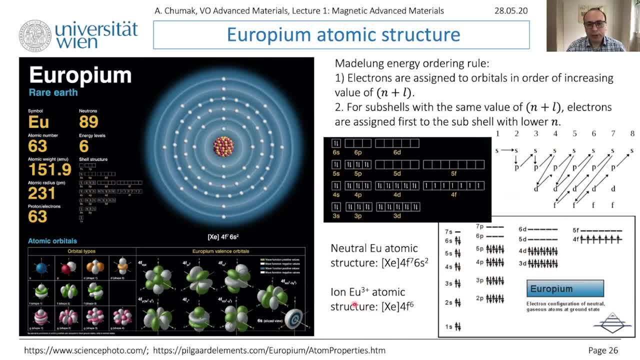 lanthanides, we usually talking about ions 3 plus. it means that out of your atomic structure you need to remove three electrons. so ionization is another question, but the general idea behind that: you first of all will remove that electrons which are usually the outer shell. 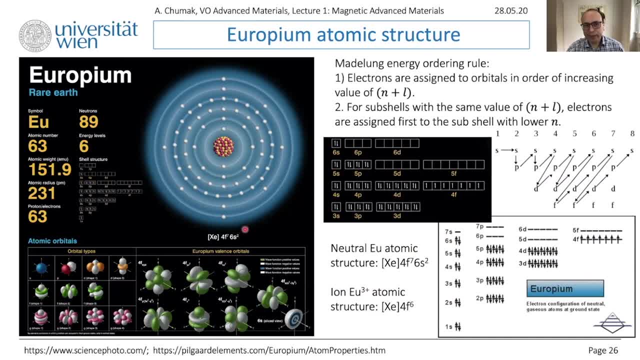 will be removed. first because column interaction is weakest. but also you need to take into account shielding of your electron by other orbitals, you know. so if you have negatively charged, positively charged, but here you have a shell which is also negatively charged, it also decreases that interaction. 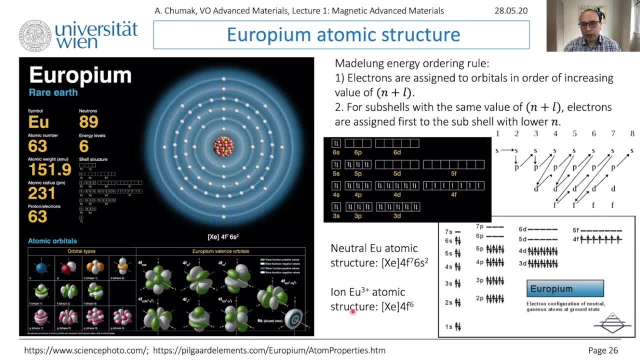 between nucleus and your electron and if, to speak about ionization, this happens, these two electrons are removed and then afterwards you start to remove electrons from 4f shell, while 5s and 5p are staying the same. good, now again i would like to make 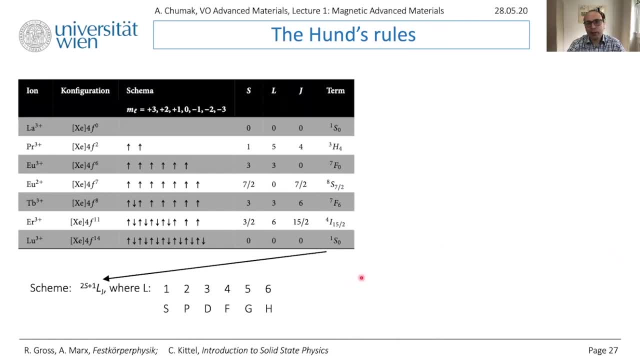 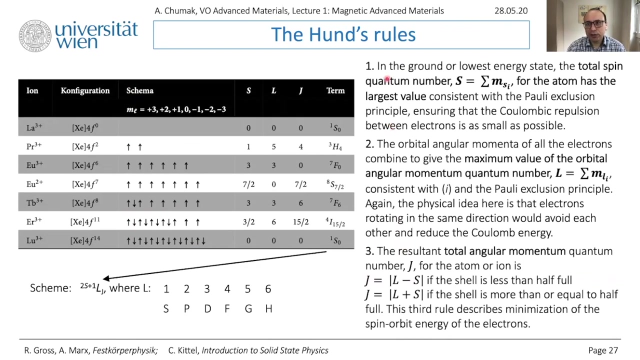 a little refreshing of your memories about the how these electrons now fill each the electronic shell because, as you know, we have different quantum numbers, ml, and the question, what will be filled first? and the answer is given to us by the empiric Hund's rule, which tells: 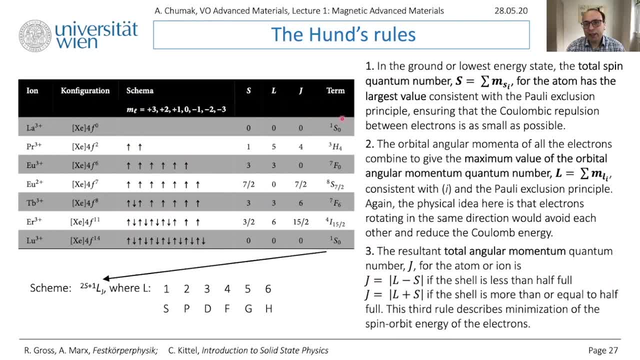 us that, first of all, we are filling our orbitals in a way that, as the total spin angle, momentum will be maximum. so it means that if you have here one, two, and in each of them you can put two electrons, what happens then? you first of all, 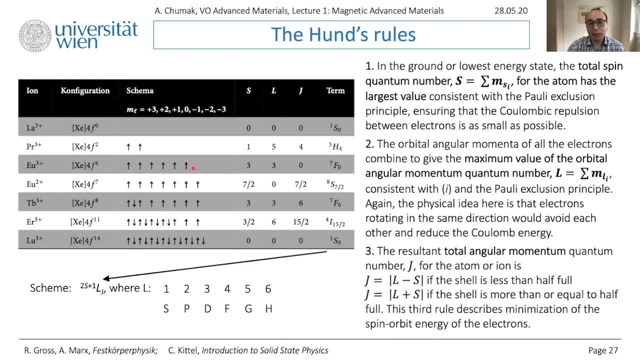 will start to put electrons y one by one with the same spin orientation, like it's shown here. then second rule tells us that we will have to maximize the orbital angle momentum quantum number l, like it's shown here. and what does it mean? it means that you start. 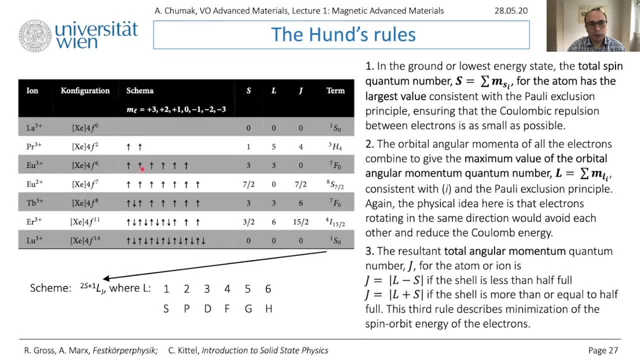 putting electrons here plus three, plus two, plus one and so on. so we fill electrons again in such a configuration and only after your shell is half filled you are starting to put new electrons with opposite spin direction and again you start with a positive, larger value of ml. 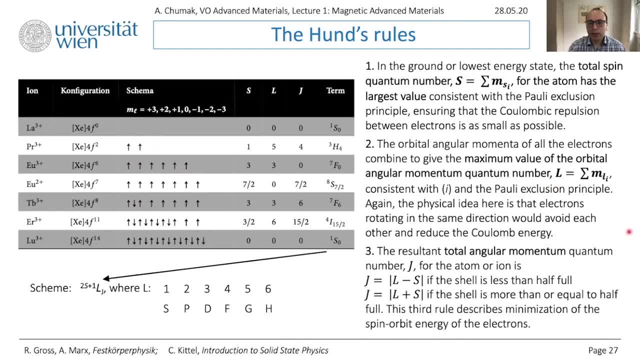 and go on. then the last rule of Hund gives us that if your shell is less than half full, then it will be a difference between orbital and spin momentum. if your shell is more than equal to half or more than half full, then you will get here a sum. 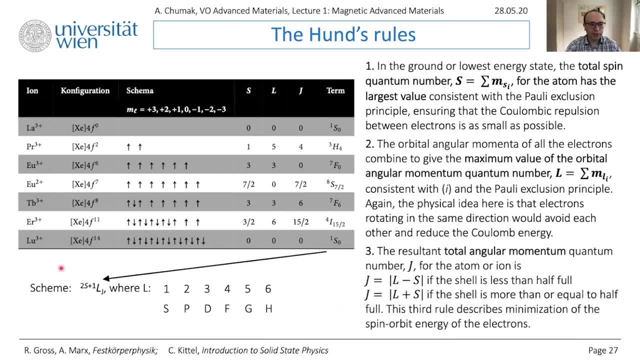 so you need to. your total angular momentum will be equal as l plus s, and so on. so that's it about the basics of atom physics. so now we know why our electrons are sitting in this shell as they are sitting, and the question is why these rare earth ions? 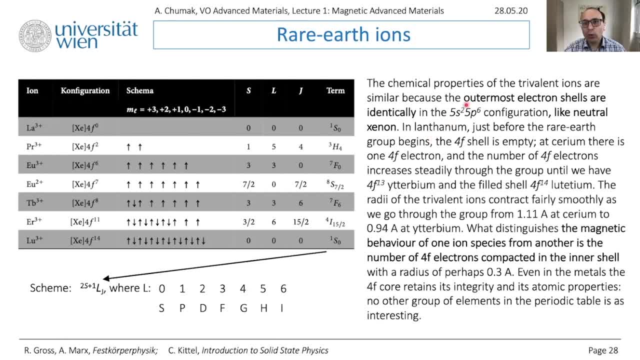 are so interesting for magnetism and the answer you can see here. the point is that all outermost electron shells which have around one ohmstrom radius are identical. so you jump from one electron to another and these shells are the same. and then chemical properties in crystallographic. 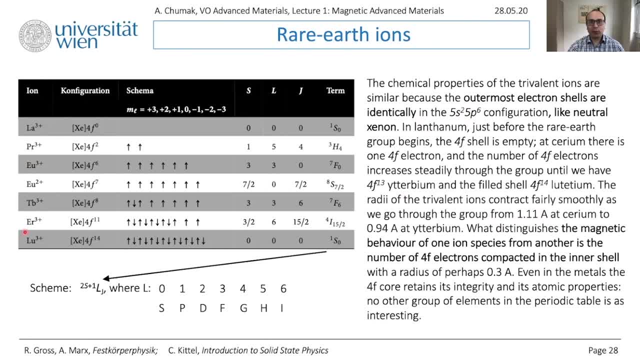 structure and so on, are defined mainly by this shell as a response, magnetic response as opposite, is given by the 4f electrons which are in the shell, and then we have a very unique situation that even if you have not an ensemble of individual atoms which you 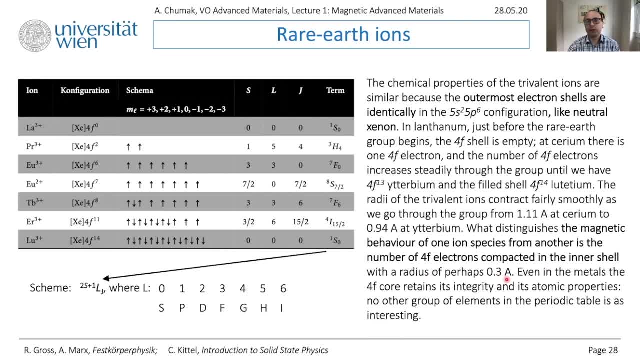 practically never can have in reality. in nature you have a complex solid body with many different processes which should be taken and interactions which should be taken with these 4f electrons. simply analyzing your solid body as an ensemble of non-interacting ions and, for example, in: 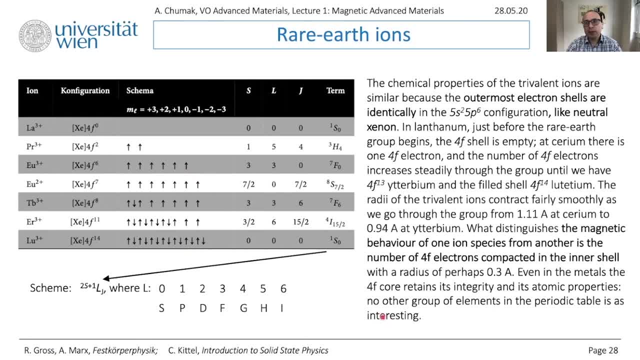 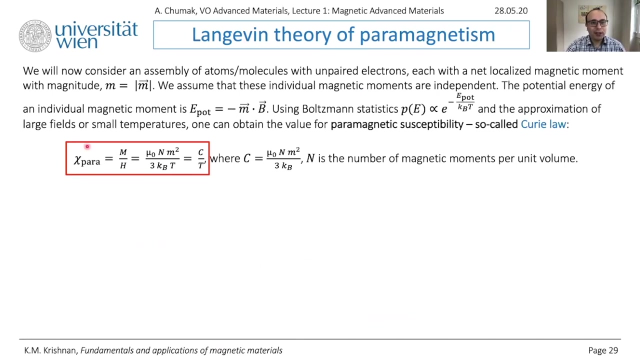 this book of cross, marx and kittel you can find nice tables where the magnetic moment of each atom is calculated theoretically and compared to experimental value. and you know, atom physics model describes magnetic response very precisely. so that's it about rare earth ions, and we are moving. 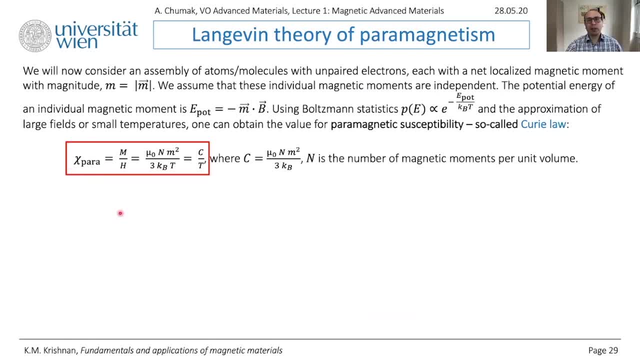 to back to the question, okay, and how to get the susceptibility of paramagnetic materials- and here we again are talking about independent magnetic moments, m and what we do, exactly like we have seen in this slide with this green arrows: we need to put them into external magnetic 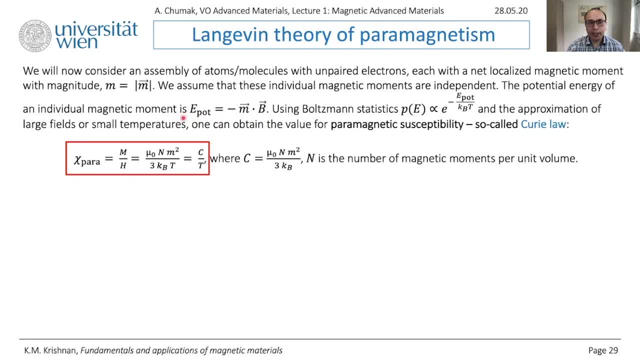 field, and then each of the magnetic moments will experience a change in its potential energy, which is found like this potential energy divided with kbt. so Boltzmann, constant temperature. so this is thermal energy of your system, and then you would have to do few mathematical steps, which 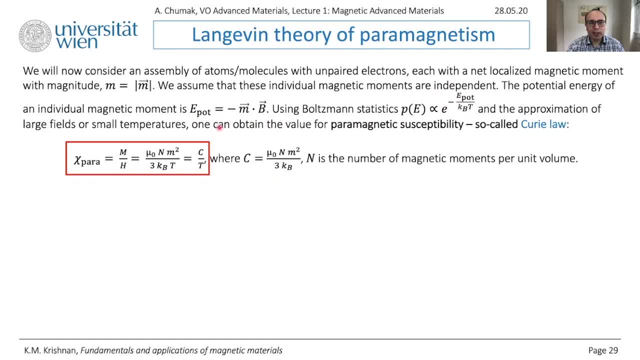 you can read here in krishnan, but here i will just give you the final result. this only comments of a small temperature, t, so as a proper formula looks slightly more complex. but this one is the most famous and it's known as krillo and its. 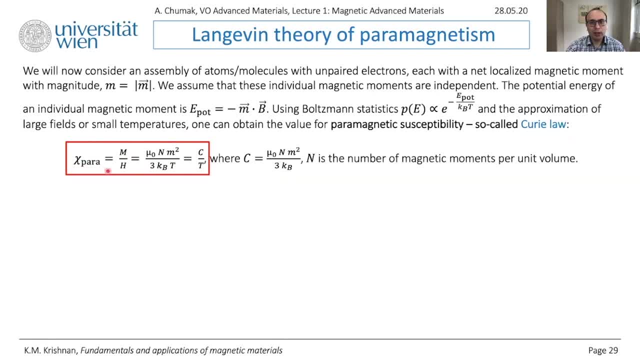 physical meaning is very simple and clear: that paramagnetic susceptibility is simply inversely proportional to the temperature. where this constant c, it is the density of magnetic moments, magnetic moment itself, squared and divided with 3 kbt. so this is such a constant which describes your material. 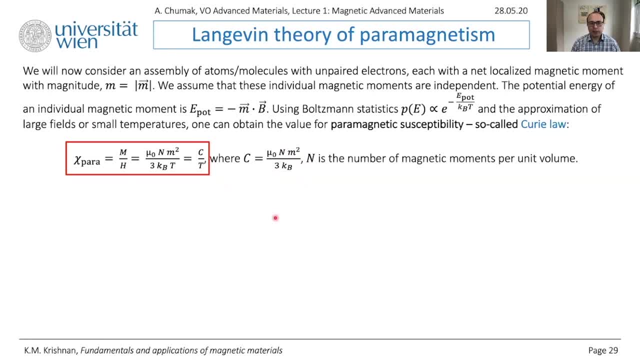 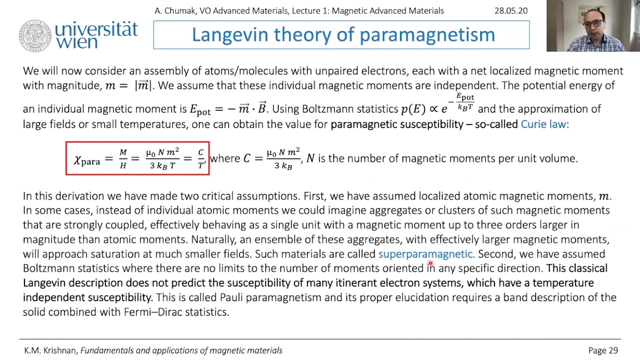 more, less. but what's important physically here is that susceptibility grows because you don't need to apply so large field in order to get magnetic order. yeah, so just few words. we will not discuss in this lecture super paramagnetism, but in some cases you should not. 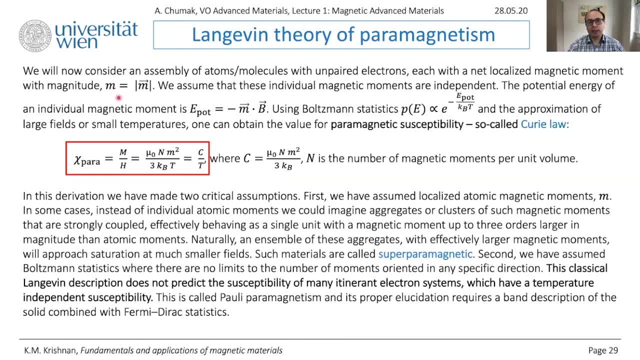 necessarily consider magnetic moments as a single atom, magnetic moments or ion. instead, you can work with some clusters of magnetization and then you will get more or less the same physics, with the difference that magnetic moments of each of your, each particle, and the susceptibility of super paramagnetism. 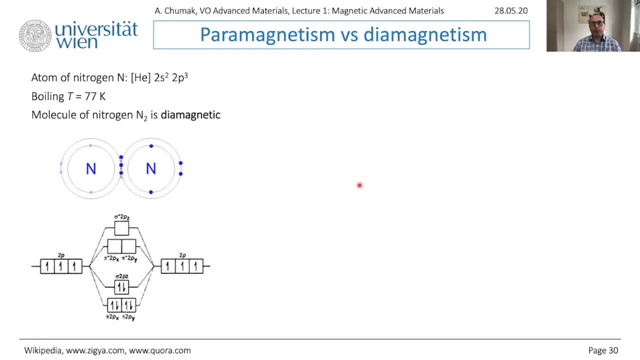 good, and now we would like to switch a gear and to give you some practical experiment, really great one from youtube. but i need to say a few words because i don't have time to answer all the questions that you may have in the chat, but i would. 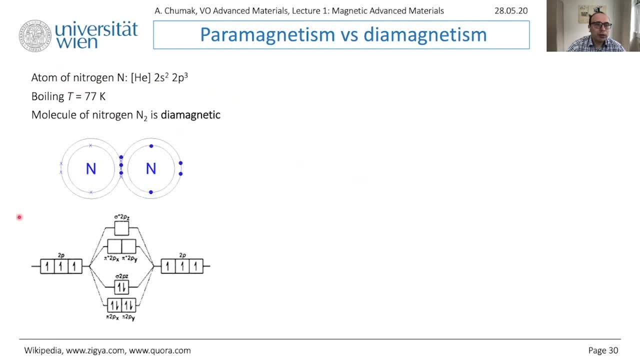 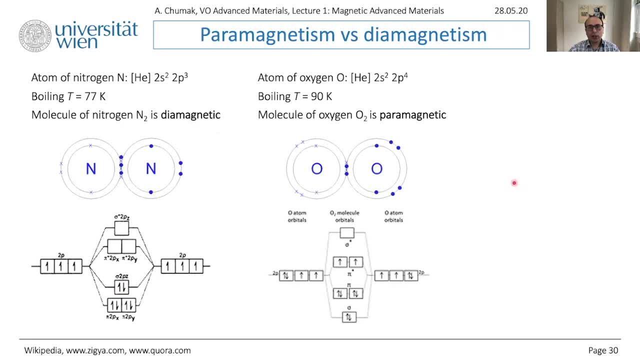 questions that you might have to answer in the chat or in the chat in the. you have here one extra electron and one extra electron here, and then, when you form a oxygen molecule, these two electrons will go up and, according to the Hund's rule, they will have. 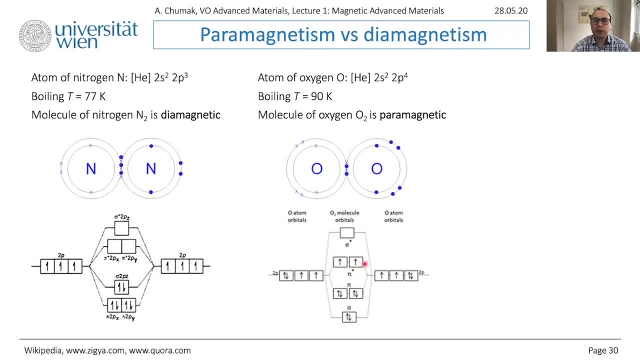 the same spin. so it means that you have here uncompensated spin, you have a related magnetic moment and it brings you to the statement that molecule of oxygen is paramagnetic rather than diamagnetic. and what's also good for this experiment, the boiling temperature of oxygen is 90 kelvin and of nitrogen 77, so it means that 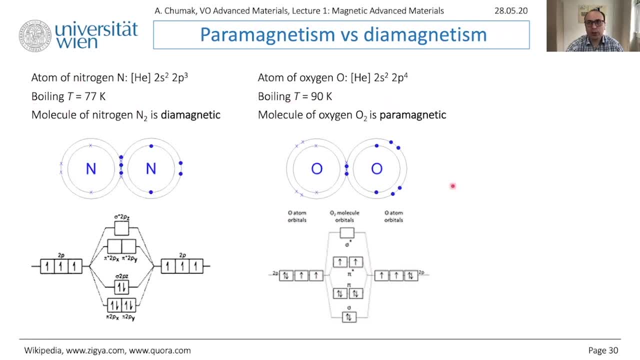 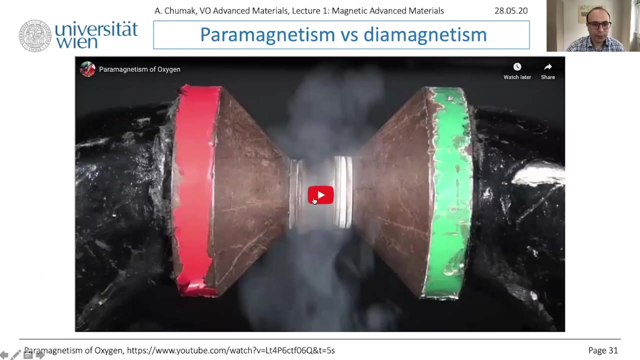 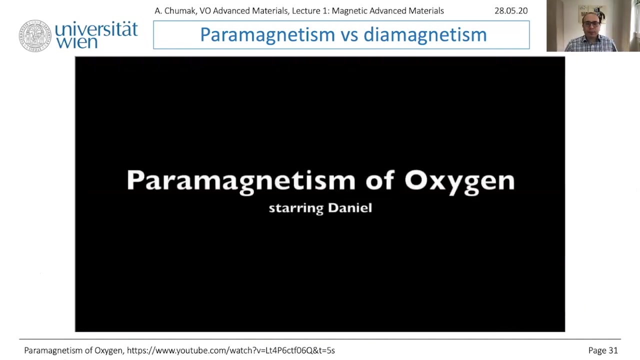 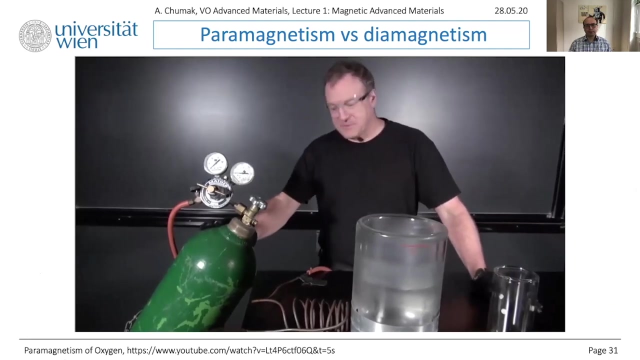 liquid nitrogen temperature is sufficient to bring your oxygen into the liquid state, and that's why we will have a look now, and let's have a look now on the experiment, and then we'll see what we can do. so we're going to take this oxygen gas, pass it through this copper coil that's immersed in liquid. 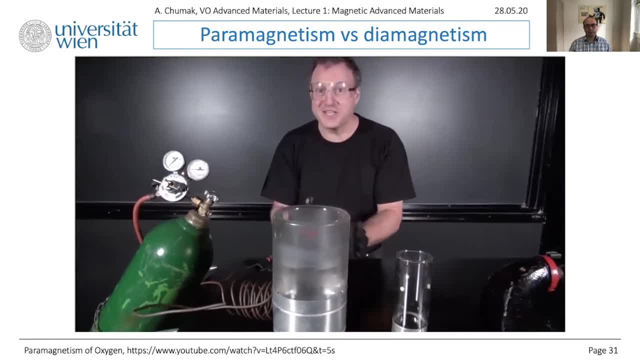 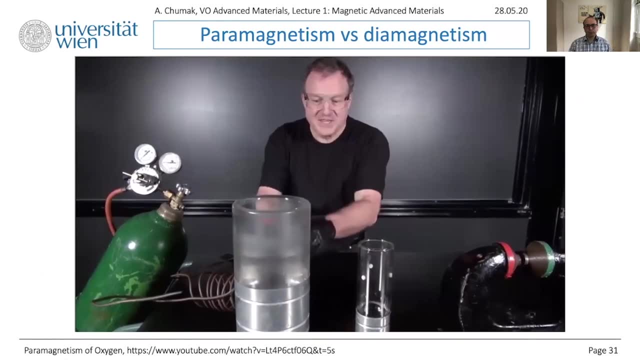 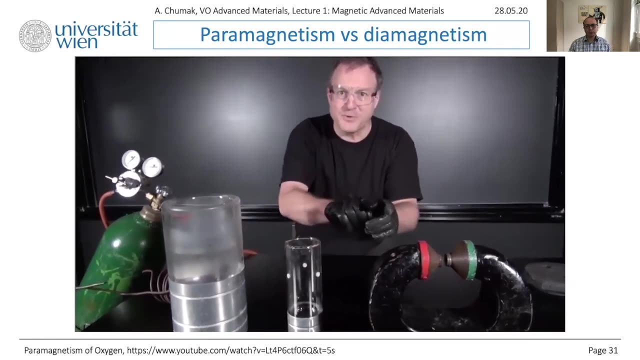 nitrogen. the liquid nitrogen will condense the oxygen into liquid oxygen, which we'll collect here in this pre-cooled doer. we will then take the liquid nitrogen and pour it between the poles of this magnet. We'll pass the oxygen also pour it through the poles of the magnet. 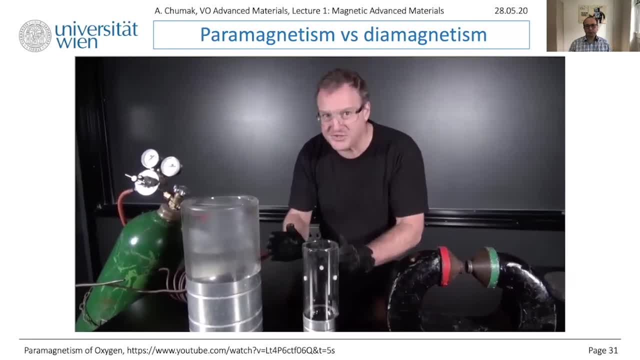 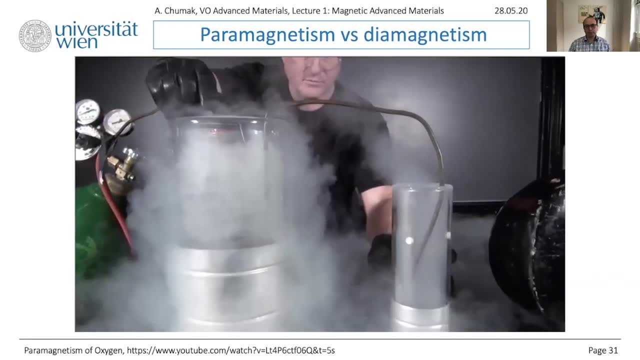 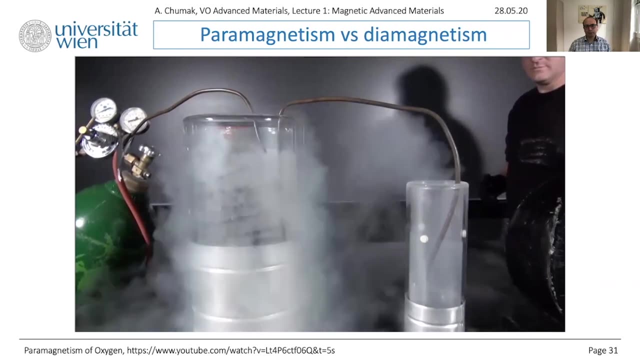 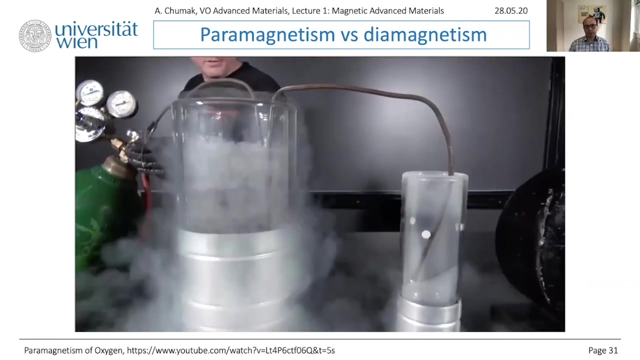 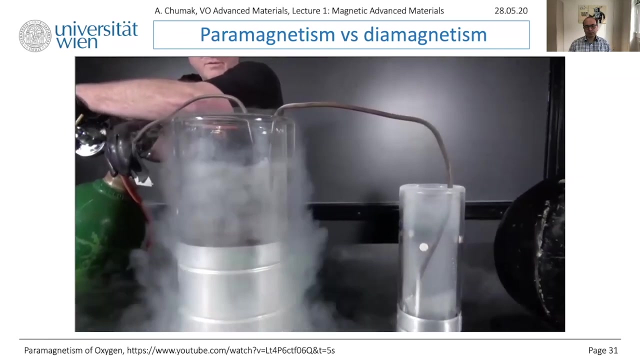 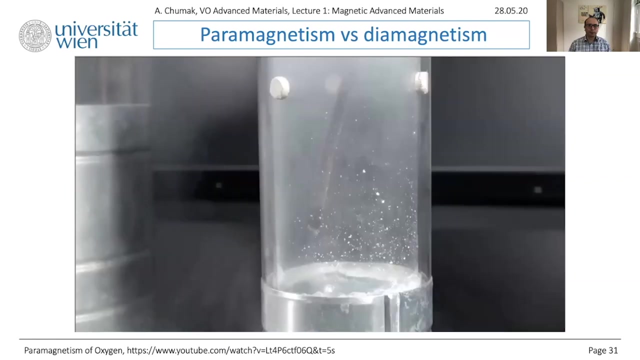 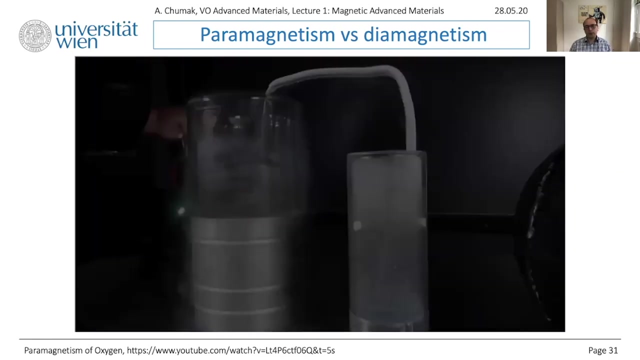 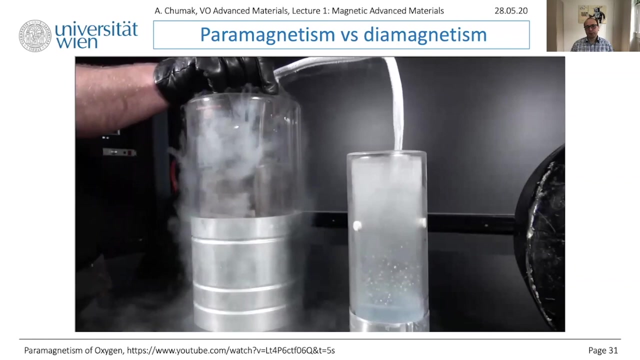 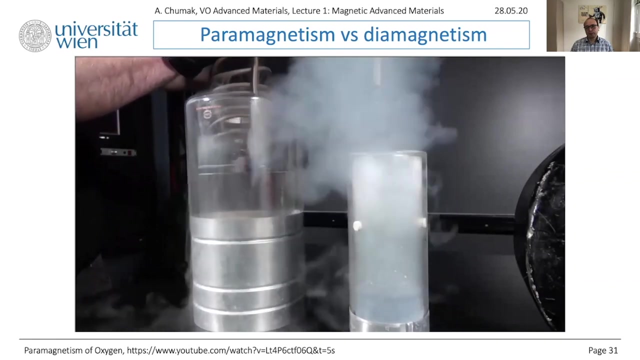 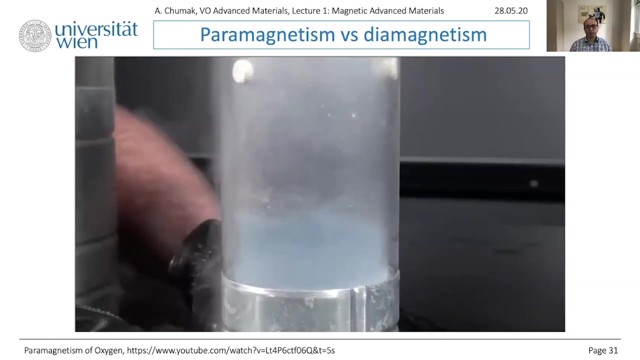 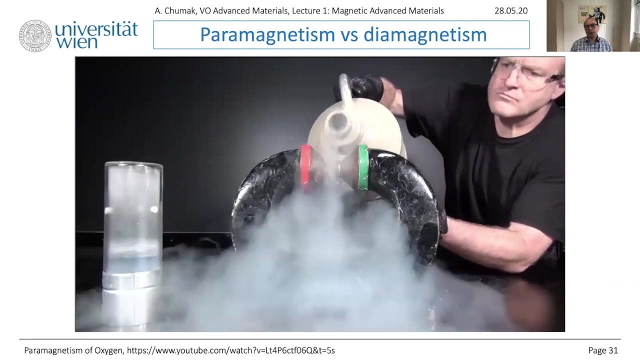 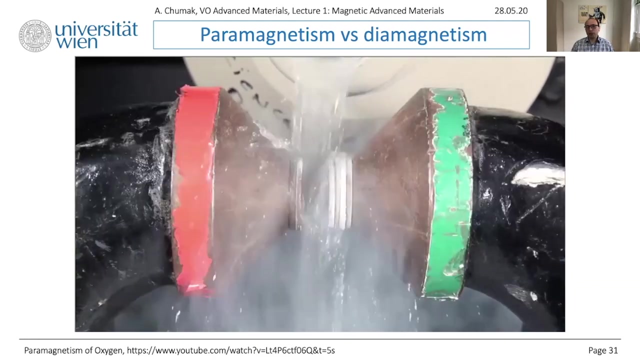 and then we're going to see if there's any difference between liquid nitrogen and liquid oxygen. This is our liquid oxygen. So this is nitrogen, which is diamagnetic. Have a look how it behaves when you put it through magnetic field. It either doesn't feel it or maybe even slightly pushes away. 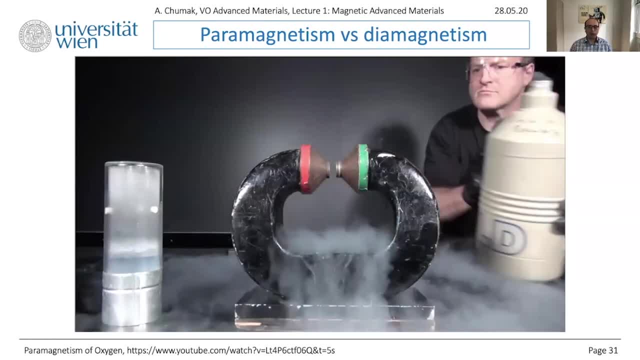 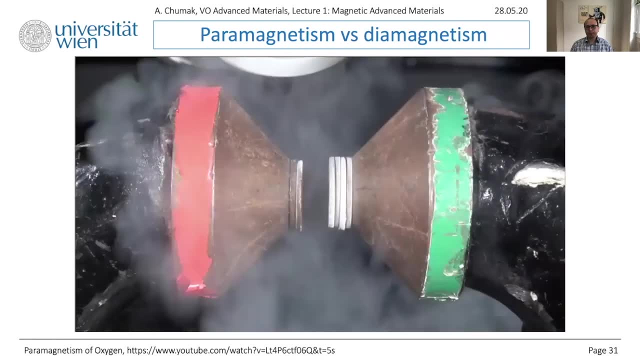 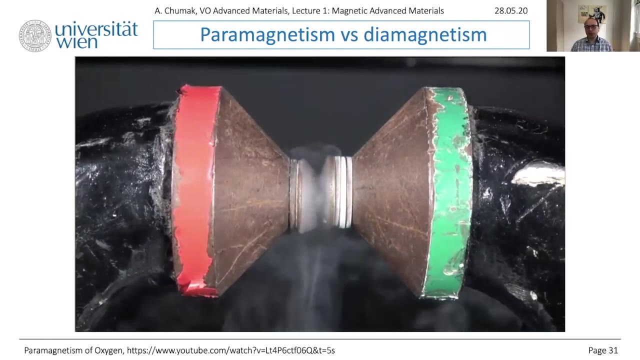 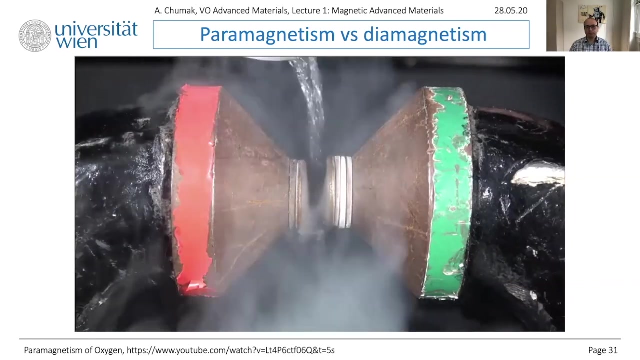 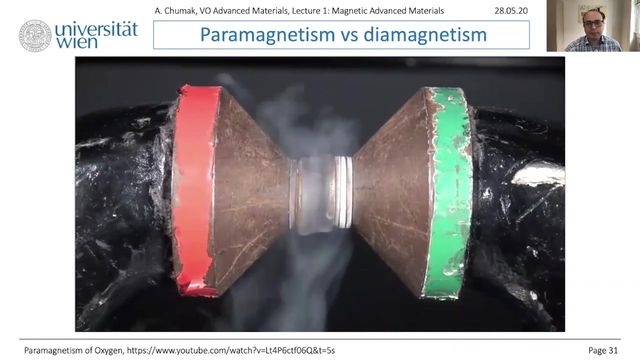 From the field or from the poles of magnet. And now let's have a look on paramagnet behavior. It's really magnetic. yeah, It's trying to stick to the poles of the paramagnet Good. I think this video is really great to feel the difference between these two behavior.